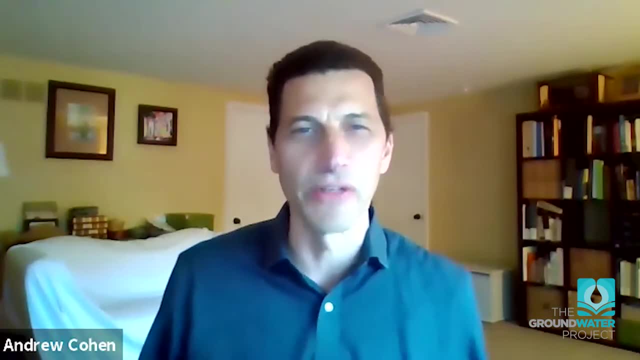 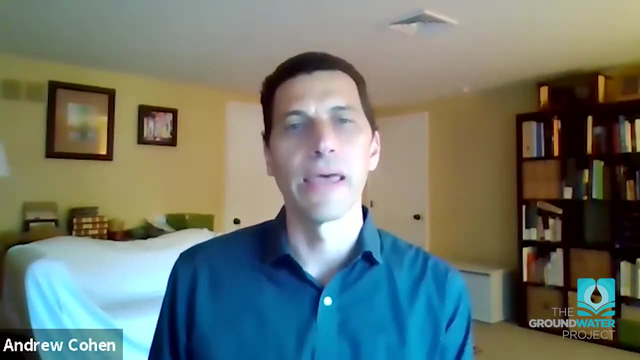 beneath. That's basically what I'm interested in. It's very interesting to try to understand what's going on underground. So that's always been my interest And I focus on site characterization, fate and transport evaluation. And of course, I do teach a class. The passion is site characterization, figuring out. 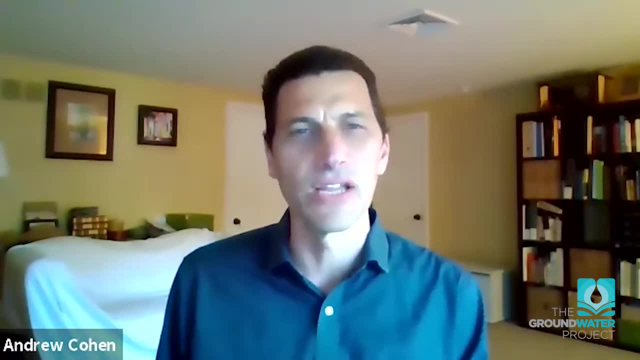 what's going on. as I like to say, That means incorporating several different disciplines. That's groundwater sampling, geophysics. So what I really enjoy doing, and what's of particular interest to me is doing, is doing a lot of work on site characterization, And I've been doing a lot of. 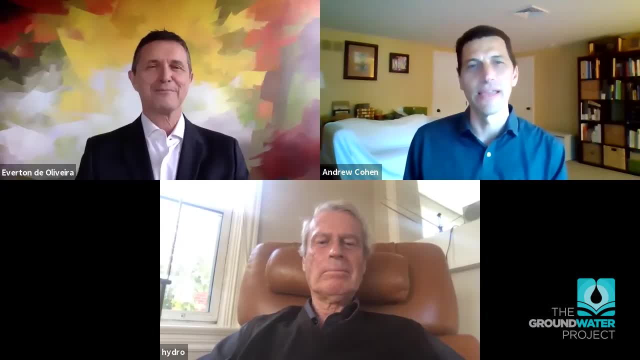 work on site and I've been doing a lot of work on site And I think one of the things that's really interesting to me is data interpretation and really integration of data, Recognizing that if we really want to understand what is happening underground, you have to pull in data from 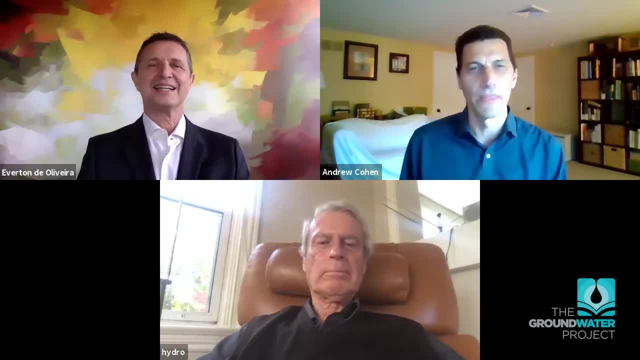 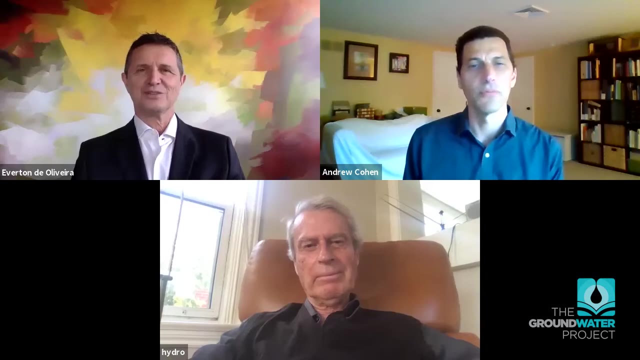 multiple disciplines and pull it all and make the story And also tell the story correctly, And that means you have to present this information in a compelling manner. So that's really what I like to do: The data synthesis, borrowing from different disciplines. I'd say that's it, John, would you? characterize me? Sure, yeah, You have a great question. Do you have a special, a special passion for hydrogeology or anything? is your passion in hydrogeology Today? anything? I think I took my first groundwater class when I was 18 years old at the University of Saskatchewan And 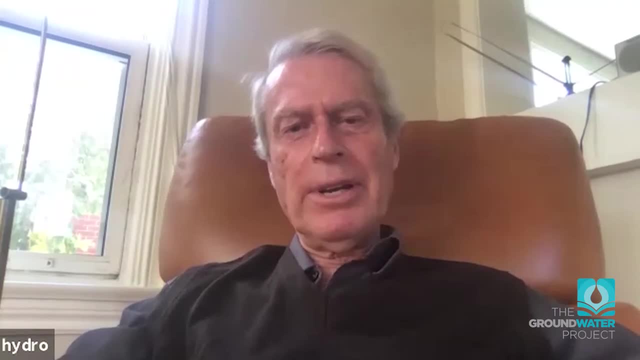 that introduced me to the topic and it seemed very interesting, And so groundwater has been my passion ever since, And I went and got degrees, of course, and then became a researcher at a university and whatnot. Research was my passion, But of course as a professor you have to do some teaching, So I taught the 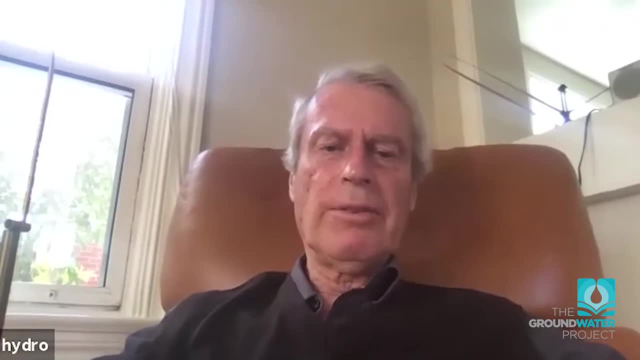 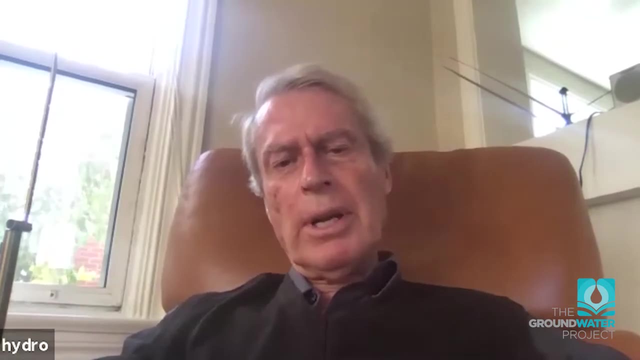 introductory groundwater class at the University of Manitoba and at the University of Waterloo for 25 years or so, And in the midst of that teaching, well early on, I realized we needed a textbook. So Al Fries and I wrote the Fries and Cherry groundwater textbook And then, in a decade or so after that, I 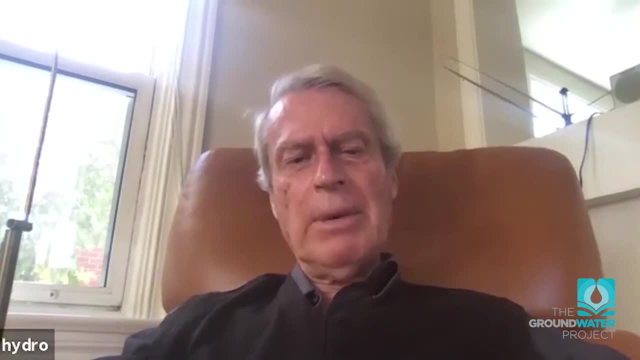 realized that students weren't learning very much Somehow. you know. first you can blame it on the students, But after a few years you have to blame it on on the professors and how we teach and what we have. I realized back then that that to figure out how to teach 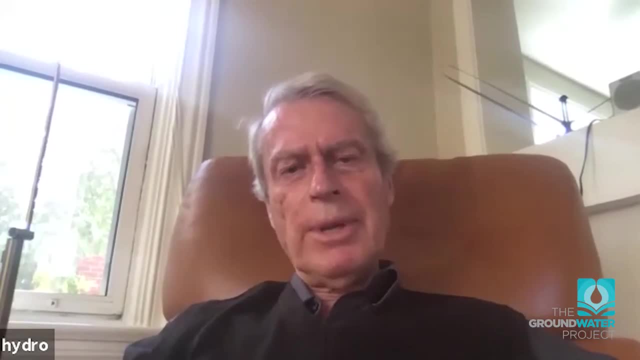 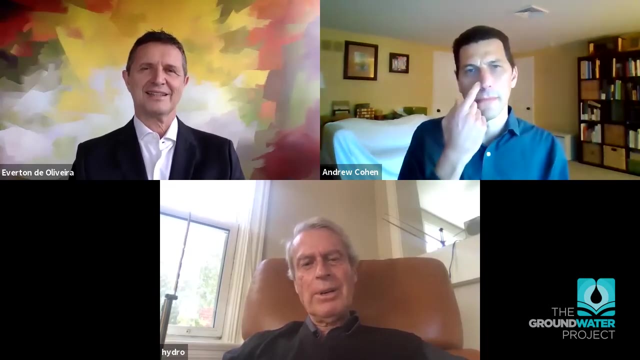 groundwater better would be a career's objective. So I did very little teaching in the last 30 years of my career. But now I've arrived at an area again where teaching and education is now my main passion, with the groundwater project- just figuring out how to help people learn about groundwater. 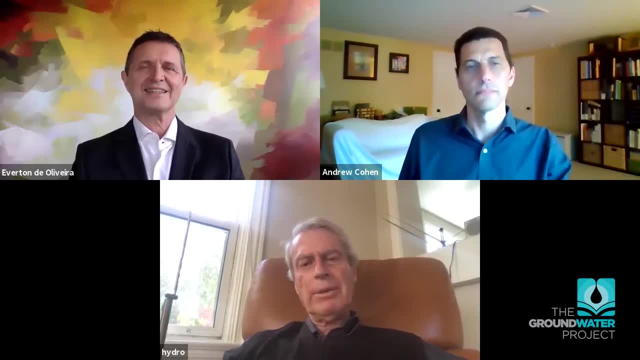 And the reason why I'm there is because I want to help people learn about groundwater, which can appear- can appear- to be trivial, but in fact, it's highly complex and needs aids to do that, And that's what this book is all about. 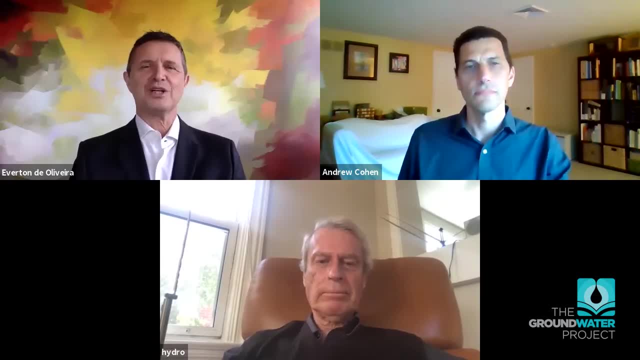 That's very good. Well, the the name of the book: conceptual and visual understanding of hydraulic head and groundwater flow. it looks very big, But the the what you do is. you know you try to work the Darcy's law and law. So for me this is an. 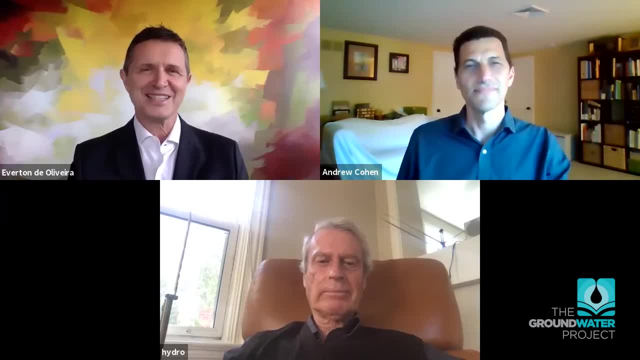 amazing too. i just loved it. whose idea was that? can you tell us how this came to to reality? i mean, i again i'm just going to kind of speak informally like we're in a conversation, yes, and that's what we are, that's right. so this started out. uh, john approached me last april uh, asking if i could. 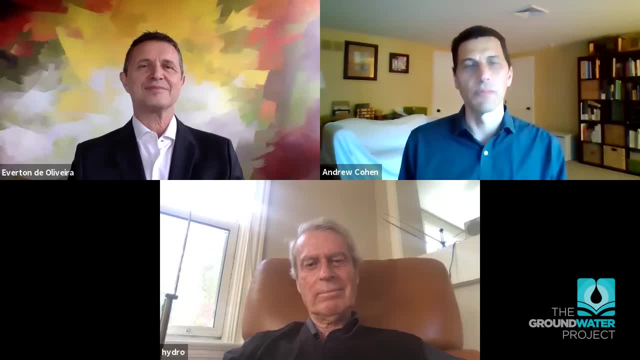 help author a book that covers some of the fundamentals and in doing that we realize that it's worth focusing on one particular area. it was both of our experiences in teaching hydrogeology that where students really get caught up or is actually at the very beginning with the most essential elements, that is, measuring water levels and interpolating the data. 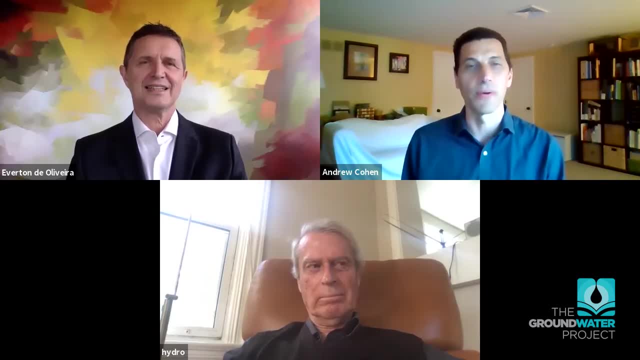 so that you can figure out basically which way the groundwater is flowing. and that's actually the greatest challenge and the way i like to to put it. you know, if you, if you don't know which way the groundwater is flowing, you really don't know anything. it's kind. 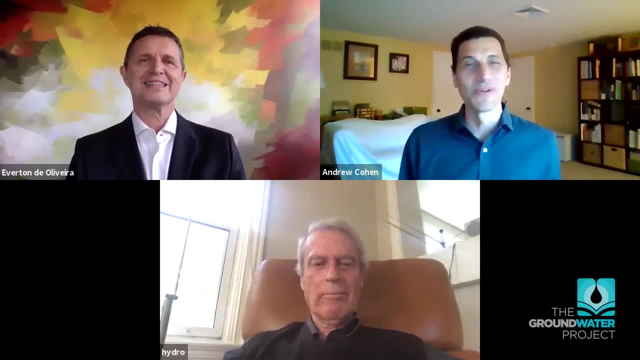 of like: if you want to study a river, if you need to know which way it's flowing, that's the most one fundamental piece, and also so if you look at some of the traditional ways in which, now, i should say, darcy's law is much more than just looking at the darcy experiment. 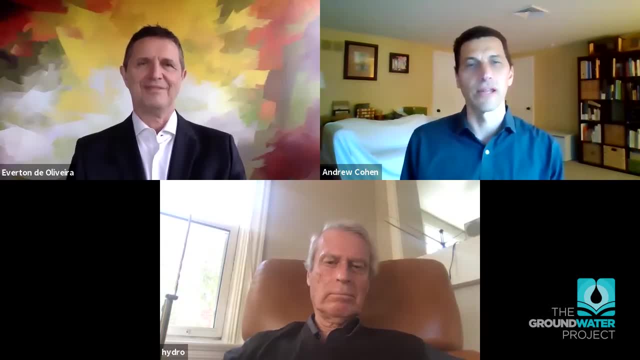 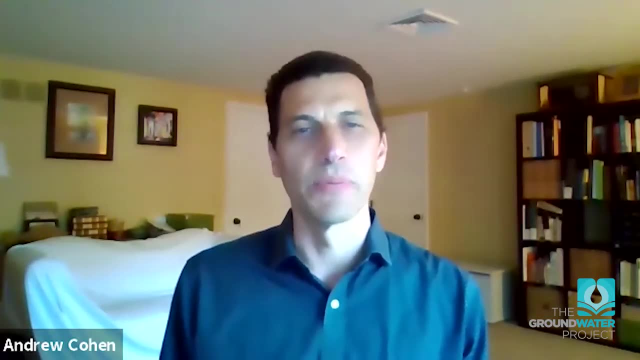 and talking about the gradient, and the flux is proportional to the gradient- really darcy's law manifests in how you, in the hydraulic gradient that you observe, in the potential metric contours that you draw, and really it's just form, forms the basis for all of that data interpretation that 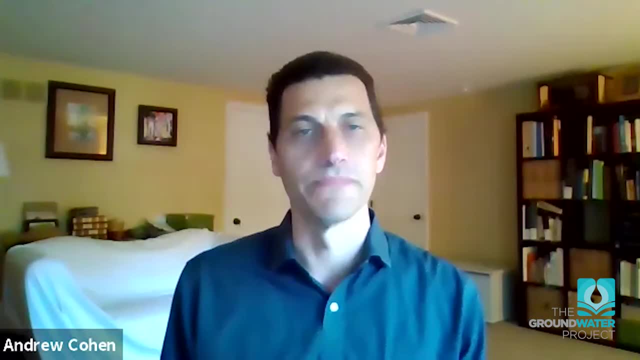 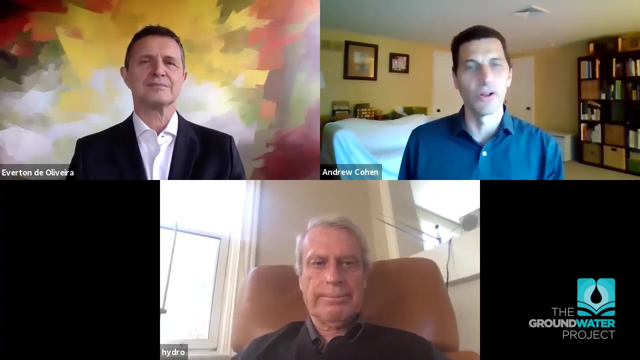 leads you to understand the groundwater flow direction mainly. so, basically, in both of us recognizing that that's where the real challenge is, we decided to just focus on this one topic because, even though it sounds like just a very straightforward- okay, get it over with, show me the equation- it's. it's quite nuanced, actually, which makes it kind of fun. 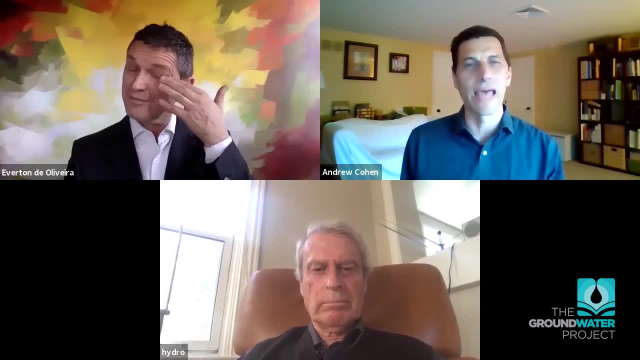 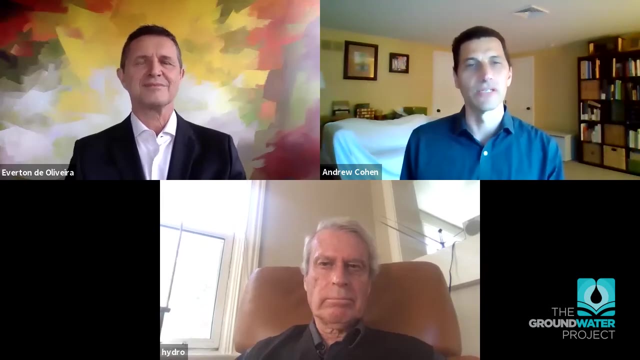 in a way, if you can pull, you know, peel the onion back on something that is usually treated as quite trivial, actually. so we called it conceptual and visual, because we're not introducing any mathematics at all except for the simple darcy equation, other than that there are no calculations. 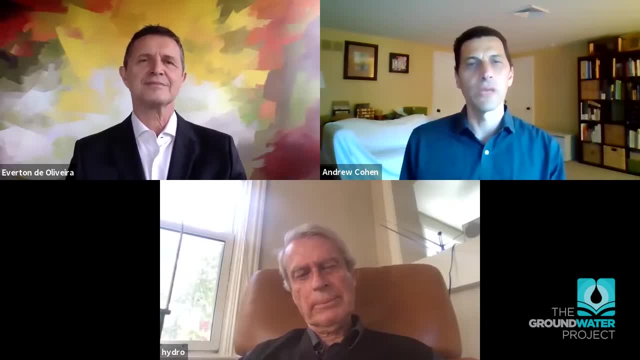 or any other mathematical presented really what we wanted. we want the learner to be able to look at data well, really interpret it correctly, essentially. but also, in order to do that, you need to have a basically conceptual idea as to how this, how groundwater- should be expected to flow, and that requires you to really understand what. 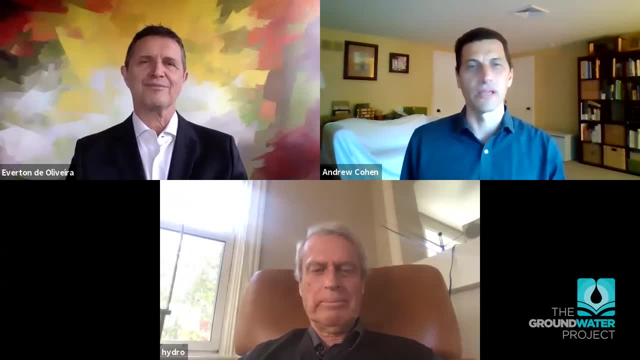 hydraulic head is all about and the distribution of hydraulic head. that's what we're focusing on. it includes much more than just discussing head. it talks about gradients, contour lines, boundary conditions- all the essential elements in what I think is a compelling and fun way. when I taught hydrogeology, you know. 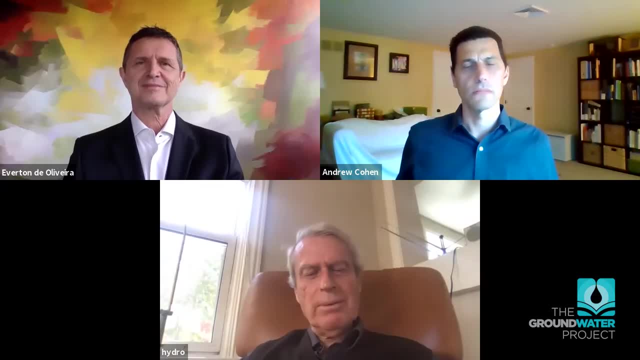 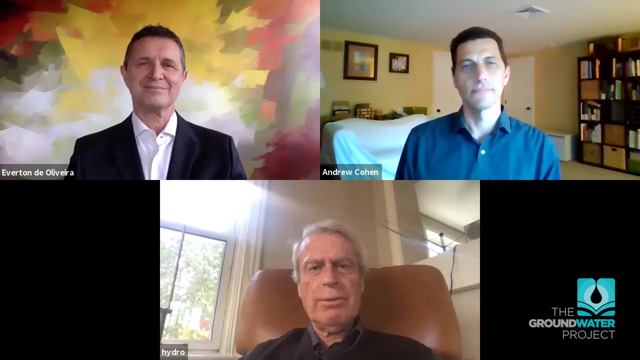 I would always be amazed at how the students after my lectures and in the exams would display a particular propensity to not be able to convert Darcy's law and hydraulic head into diagrams. and we professors, we usually gloss over that in a lecture or two, like it's just too. 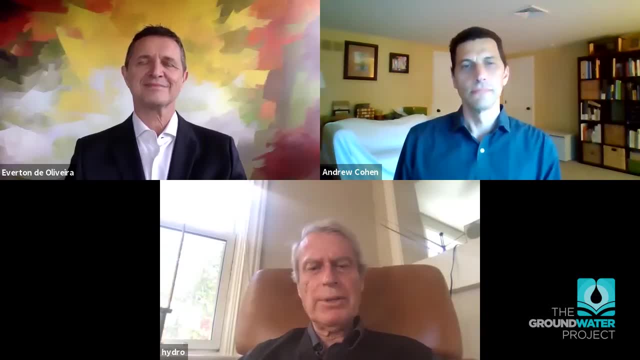 trivial. so we move on and we spend a lot of time on equations and all of that stuff, and so Andrew and I got together to narrow the subject and actually it took us several months to get the subject matter narrowed down to just basically this, what it is. 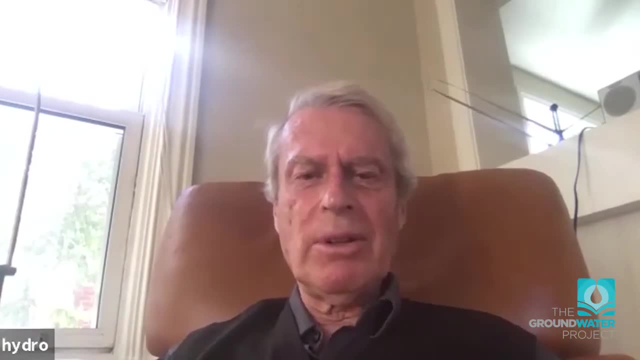 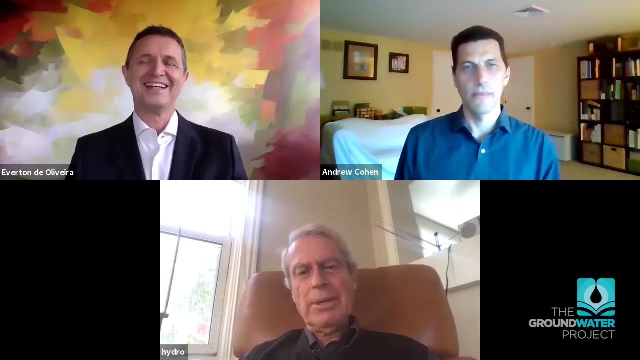 is, and i really invite the audience out there to have a look at this book because it's- i think it'll be- the most surprising book that anyone will look at. uh, yes, that it. it delves deeply into something that seems to be so simple. uh, andrew has a particular talent for uh- for drawing. 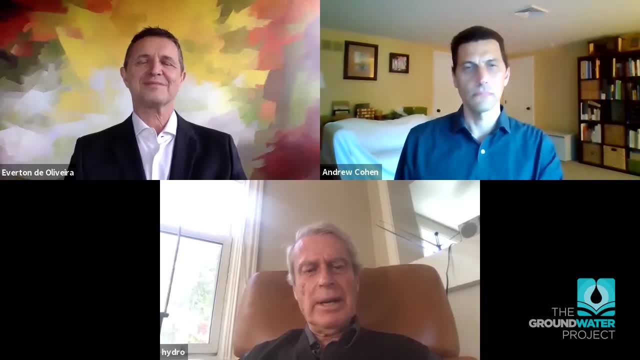 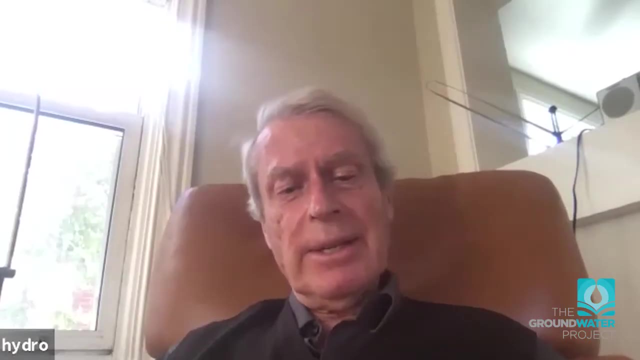 figures, uh, that are correct, uh, and yet, uh, simple to look at. uh, and as we worked our way through it- and andrew would work things up and i'd make some comments- we added more and more figures and then little problems, and i think that that, as a professor, any of you out there across the world, 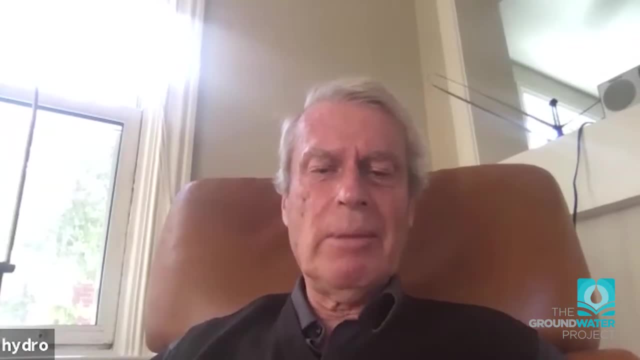 when you get into this, i think you'll look at some of these figures and you'll actually have to ponder them. some of them, i looked at them and- and you know it took me a few minutes to kind of get myself sorted out- such as the kind of the intellectually intriguing aspect of the most 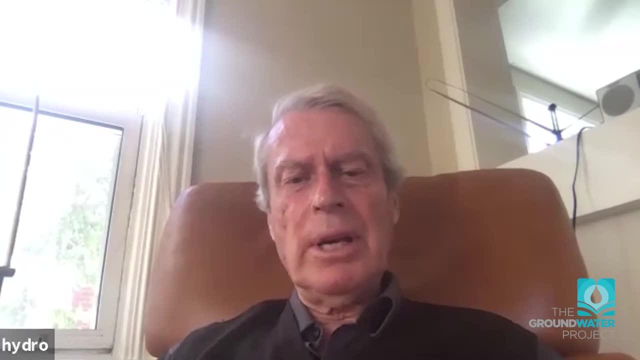 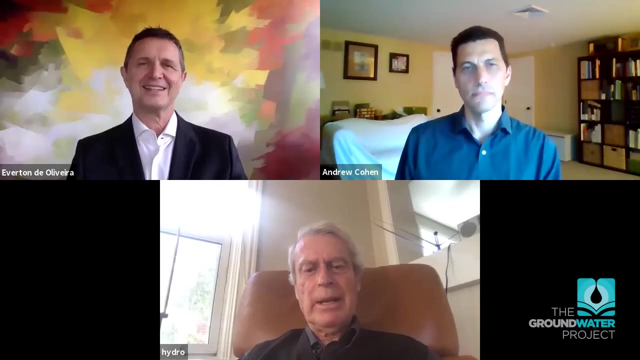 interesting uh and and uh. in fact we're not done. there's more to come on on how we can arrange little figures to see if we really understand. and the problem with conventional textbooks is you can read them and you can do a few problems and you can think you understand it. yes, the beauty. 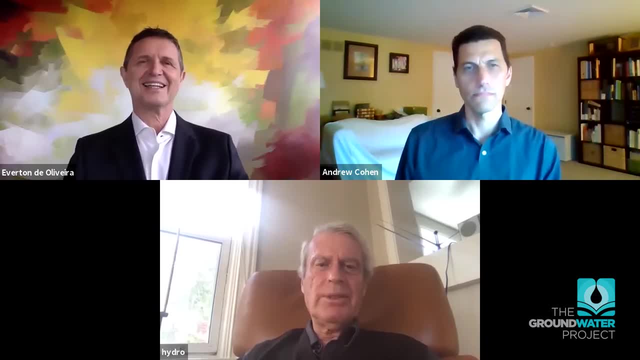 i think of this book is it continually tests you to see if you actually do. and i think, like everton mentioned, he enjoyed it and i certainly enjoy looking at the figures because they're they're little puzzles, Puzzles in the context of nothing simpler than Darcy's law and hydraulic head. 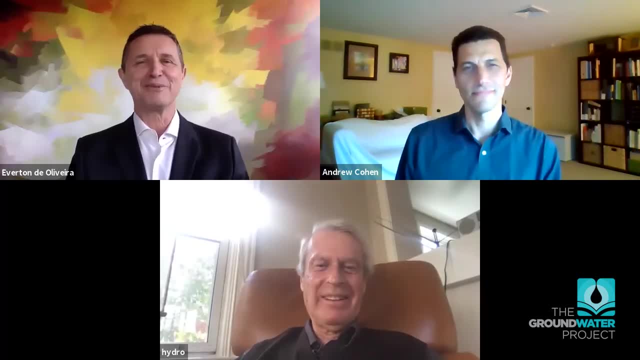 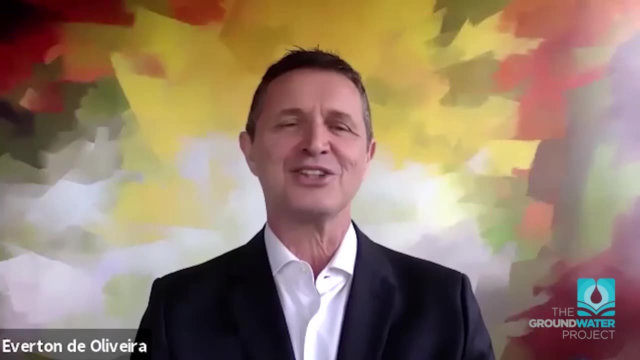 That's true. that's true. Actually, the book presents Darcy's law to exhaustion right Upside down, inside out, without actually exhausting the readers or students, right, And I believe that even experienced hydrogeologists might give it a try, like a Sudoku. 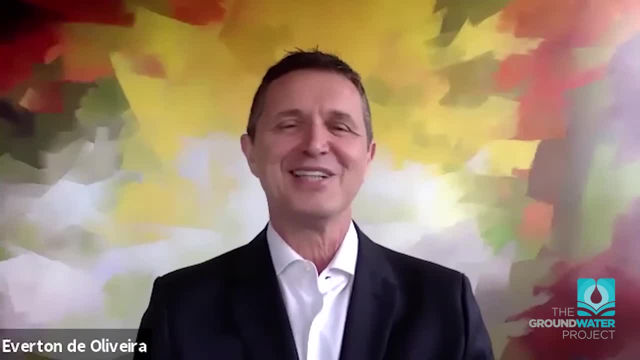 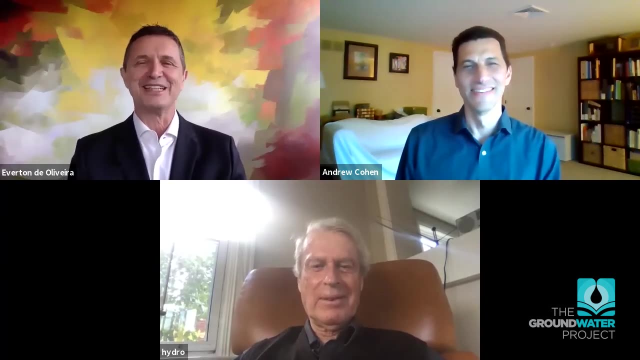 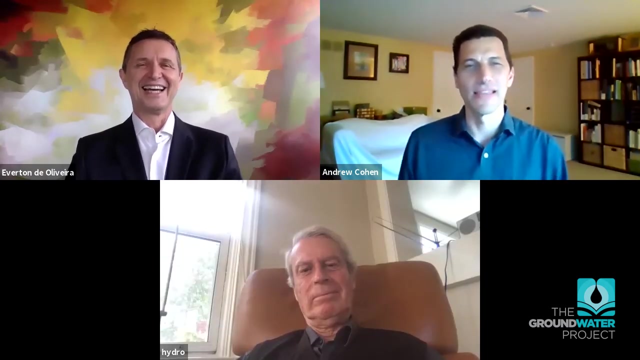 entertainment-like tool right To test their skills. How is that possible? What do you think about that? Because I think it's fun to try. I tried some of them. They're quite interesting for sure. So I'm really happy to hear that That was really the intent and that speaks to the 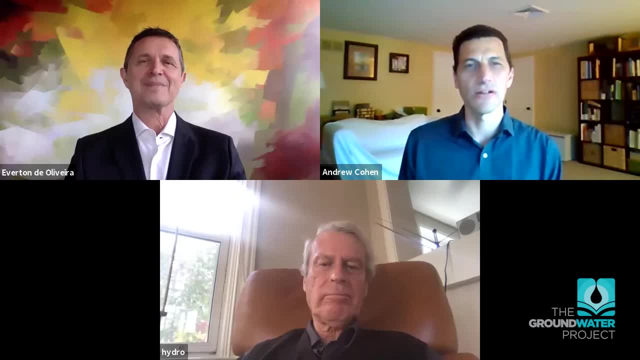 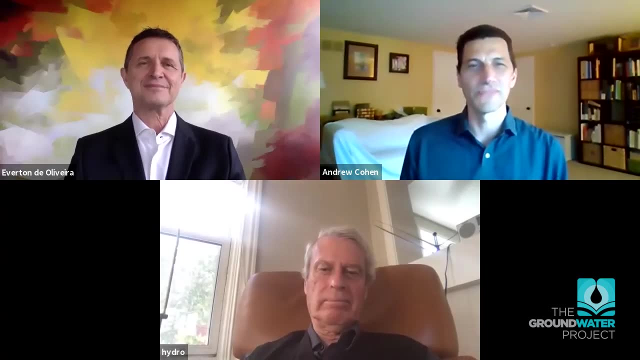 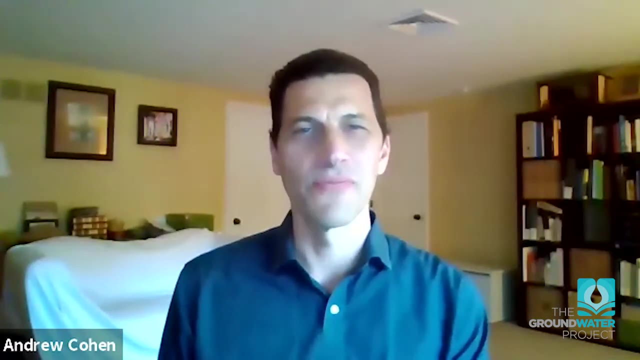 importance of understanding the subtleties that are embedded in Darcy's law. We typically think that it's straightforward to interpret water levels in wells and we draw some contours, but there are some really subtleties that you need to consider if you want to do it right. That's really what this is aimed. 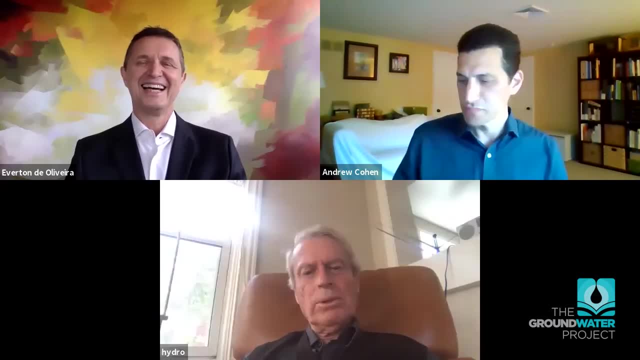 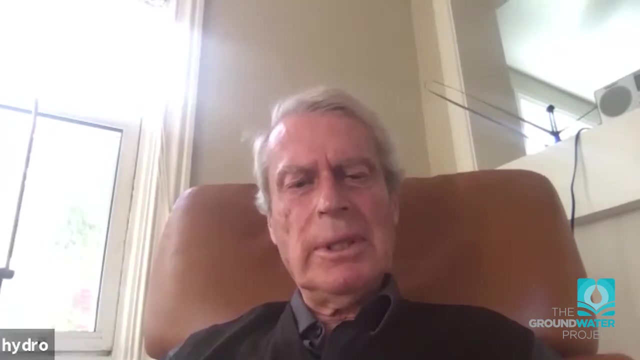 at. It's aimed at understanding the fundamentals. So Darcy's law is a little equation, the simplest of all, and hydraulic head. And hydraulic head is basically an elevation that represents energy per unit weight. But this book takes those two simple things and it converts them to visuals, Visuals in 2D, basically, And that's. 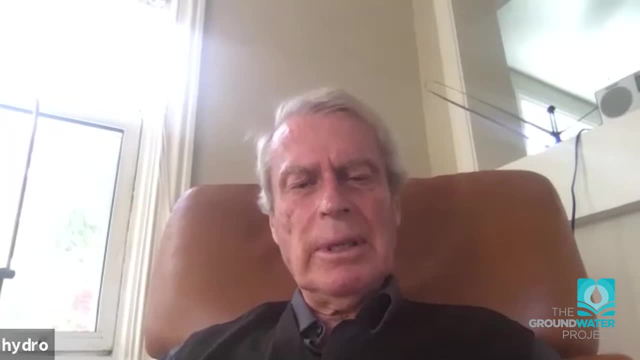 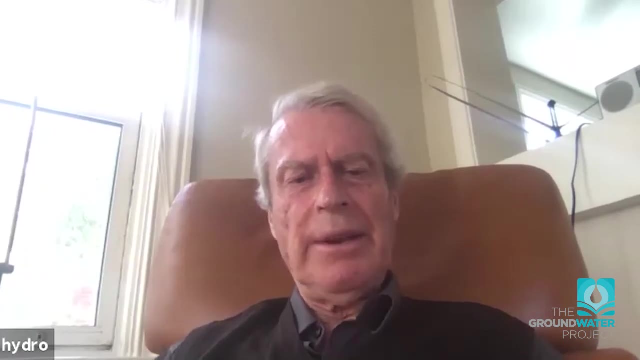 what practicing hydrogeology is all about. You know once you're done your education, what you have is data staring at you. The most rudimentary data is head and K, And so when you get out in the real world, your employers or whatever, 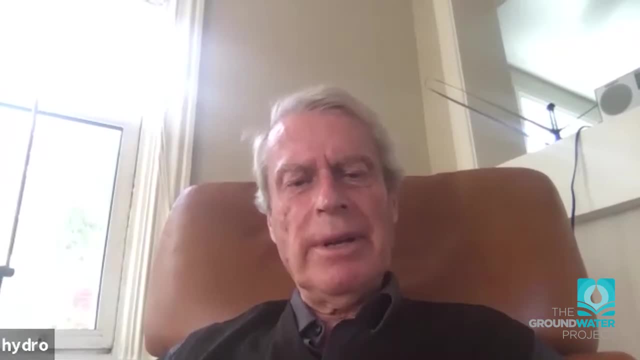 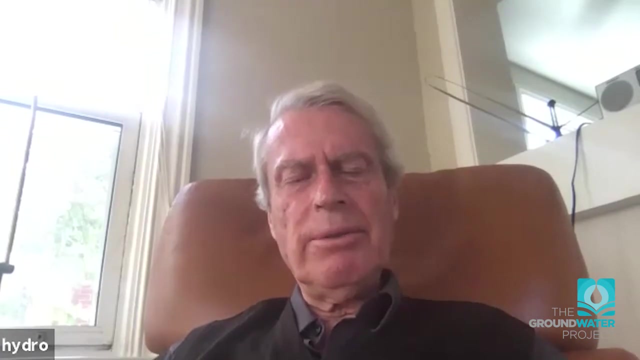 want you to explain the meaning of what head and some K information is trying to tell you, And in many cases all you have is head and you're trying to figure out hydraulic conductivity. So I think the point of this is to develop an intuitive feeling by the student. 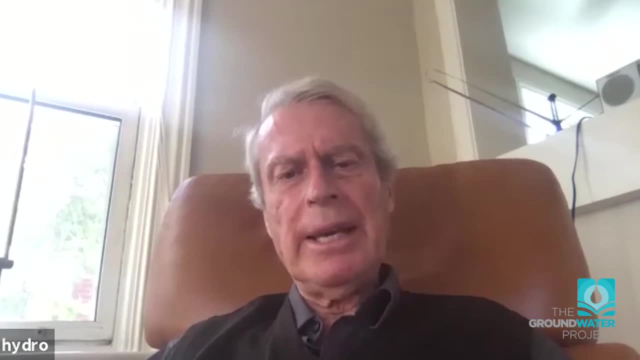 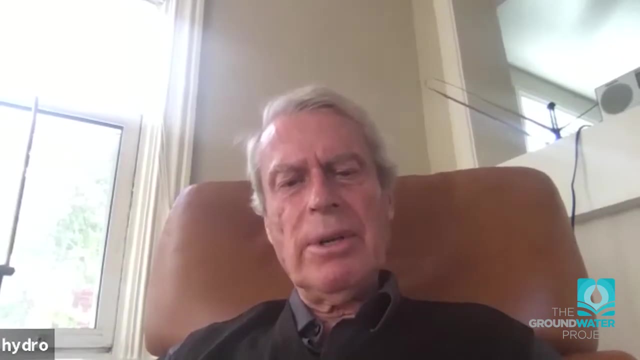 and you're, you're, you're picking out the old Time lapse True Sons games or Eddie від the old Satan board about is- is this thing we're learning as a computer programmer because we're living very much in afun and at being at personal time, for how do we improve ourった? 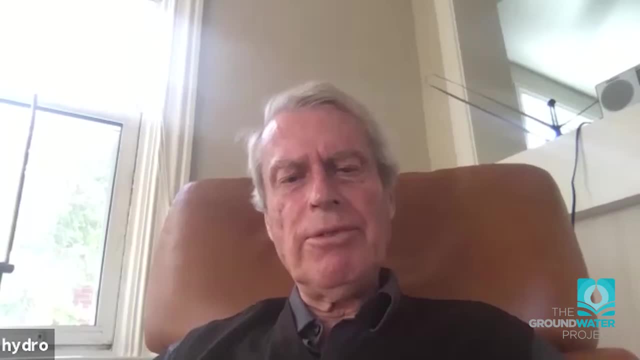 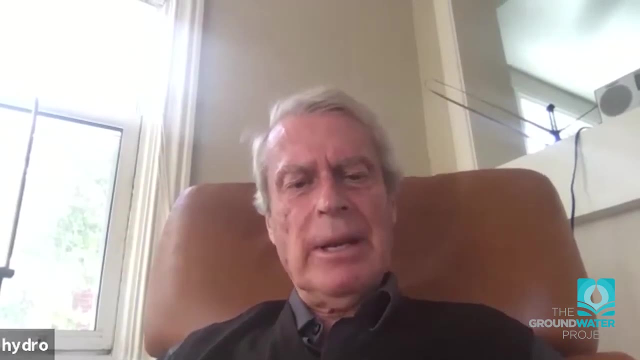 ツ to how to convert information in the form of head and K into a visual expression, into a sketch. So the little figures that Andrew's drawn here are sketches, Sketches that he's done marvelously in PowerPoint. that can the 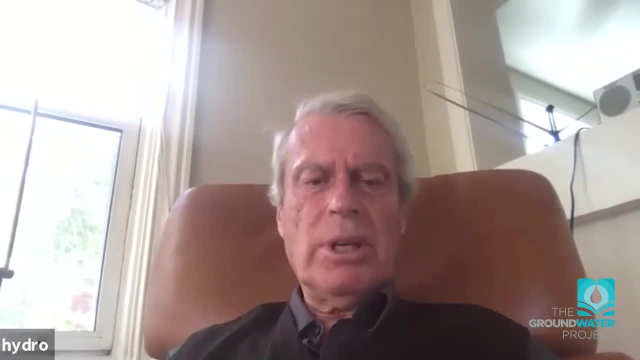 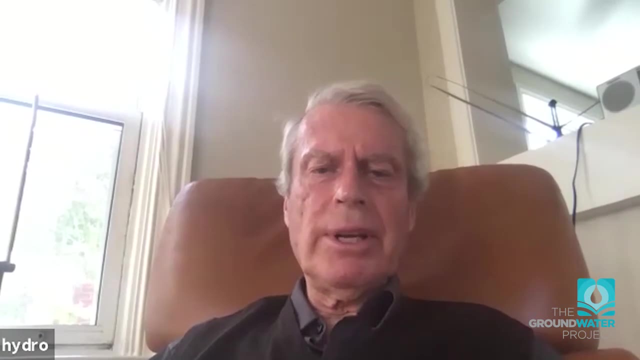 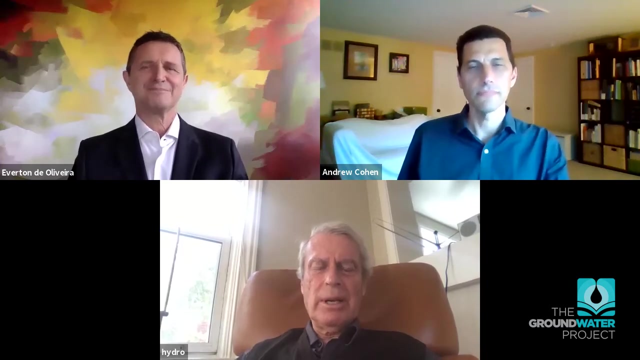 A- A- ensa prayed to give an interpretation, so the this book then leads you from the simple stuff head and k on into challenging the reader to convert such data into interpretations, and that's what hydrogeology is all about, and that, in essence, is why the educational student system, in fact, is failing. 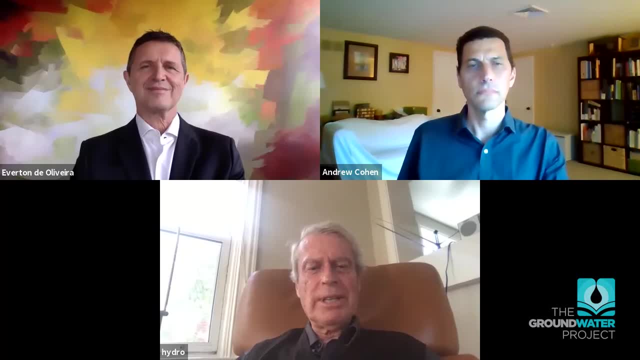 the students. i failed the students when i was attempting to teach. the freezing cherry book failed the students because it glossed over this topic in two pages or whatever. and that's the way textbooks were back then. you know, the publishers only allowed you 600 to 500 pages. but now, with the electronic 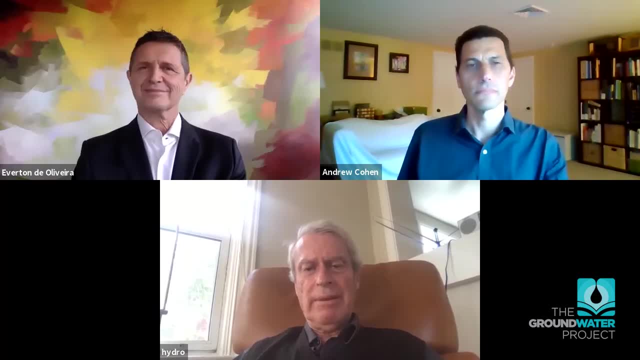 media. we don't have the excuse, then, of brevity, so we can, we can work over this topic right down to the last detail, and, of course, there's always another diagram that you can add to help the understanding, and andrew and i now have another dozen or two diagrams in our minds that could be. 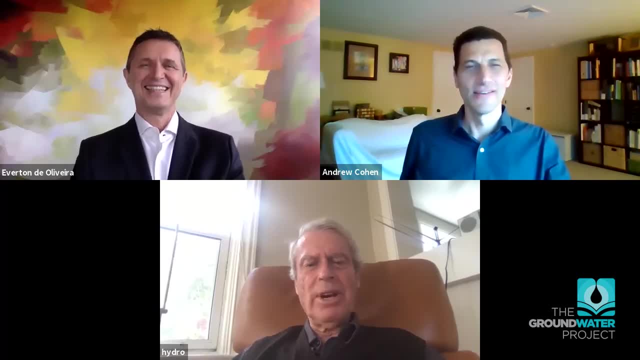 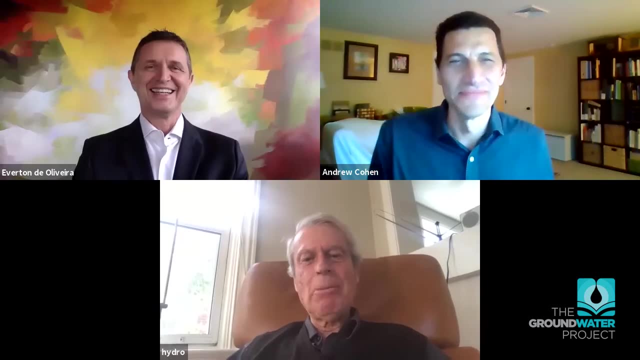 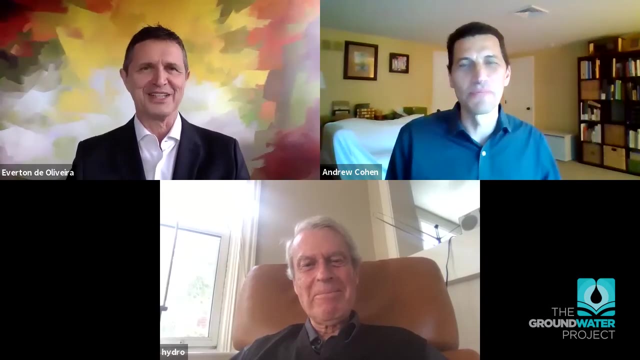 you know you could say: how could you add: you've already got 40 on this simple topic. now we continue to add: no, yeah, and it's so much fun, and it is true. i was here here thinking sorry for interrupting you guys. you're thinking because i- i usually have, uh, had problems with people. 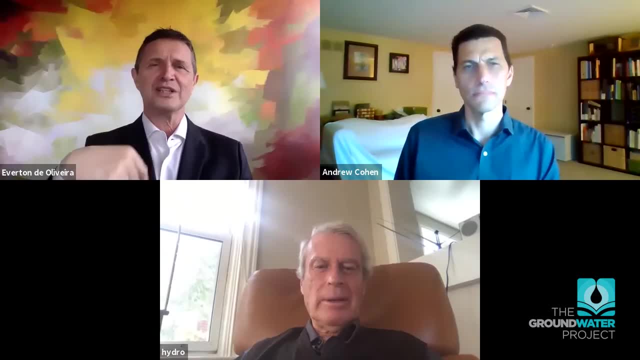 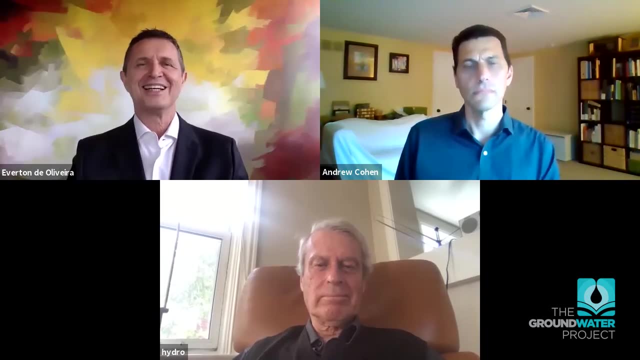 when starting in my company to to they go and they have to to to do the, the contour of the potential. you know the potential lines on the in a field on a map, right, and first thing people want to do is go to a surfer or some some software like that that has no idea what goes on with. 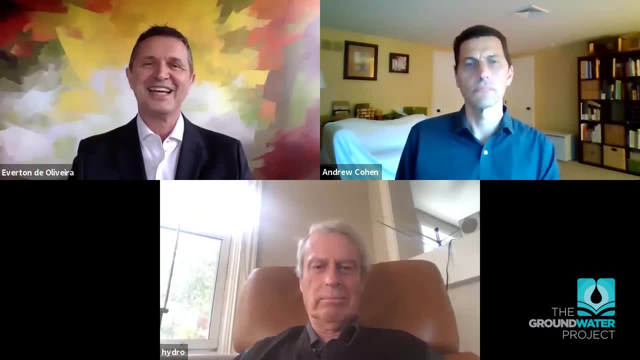 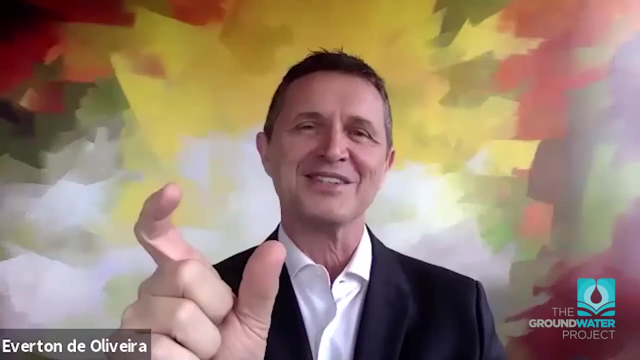 groundwater and the physics of hydrogeology and comes up with the weird math. it has nothing to do with the real world, right? and then the idea is that you have to interpret the, the potential of, you know the, the head from between two wells, so you can put the map in your head first, so you 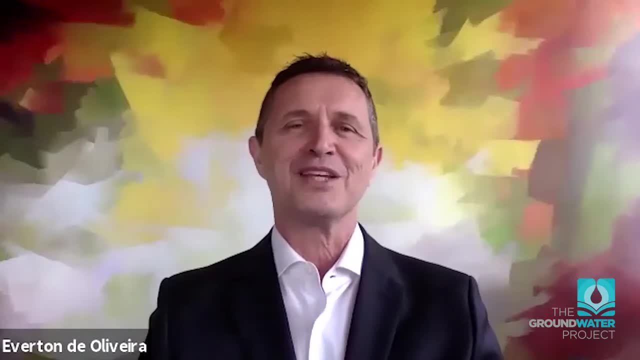 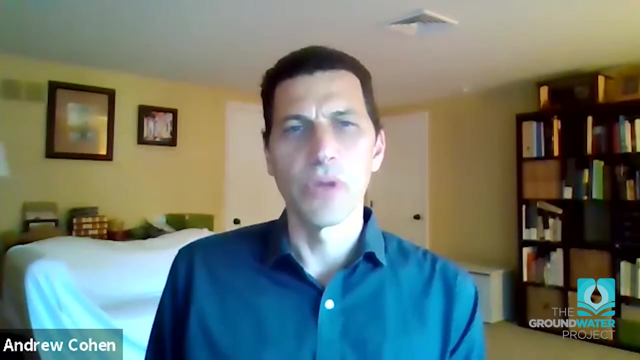 can draw the contour. so that's what i see from this book. you can. you can work in several ways before you get to the final map, because you have to understand the flow before you go. is that, is that the intention? but that's, that's certainly, that's that's correct, and i just want to when. 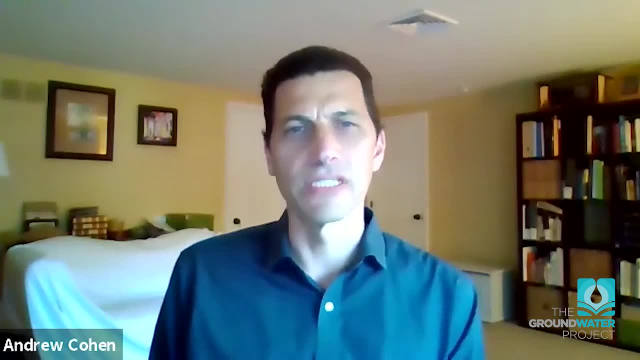 you asked about the, the simplification or how this is made intuitive. one thing that i think we can do is we start out by demystifying this notion of hydraulic head. you look at some of the traditional textbooks and even how it's typically taught. you break it up into pressure and elevation. 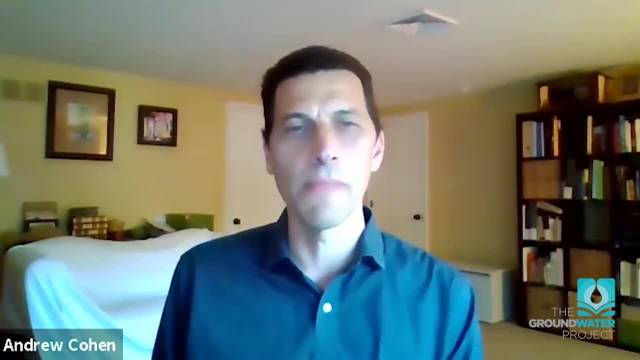 you talk about density and gravity and really what we make clear over and over again is really all that matters is the elevation of the water level in the well, and we keep on driving that home and we use that to formulate these problems. and the question is: how do we use that data? forget about gravity and all that other stuff. 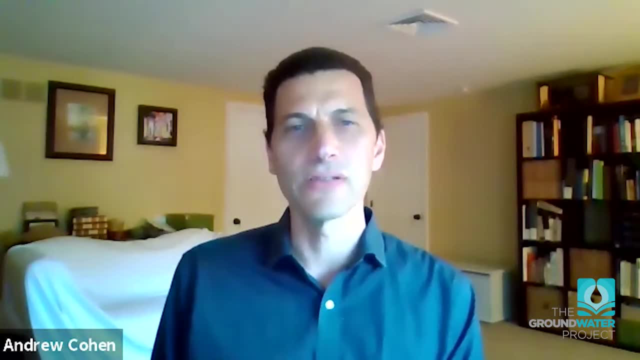 how do we use those water levels and, given certain kinds of scenarios, geologic scenarios that you would encounter, what kind of flow directions would you expect to see? and that will guide the reader: how to actually interpret data in the field as, as you noted, you know, you cannot simply just triangulate data. 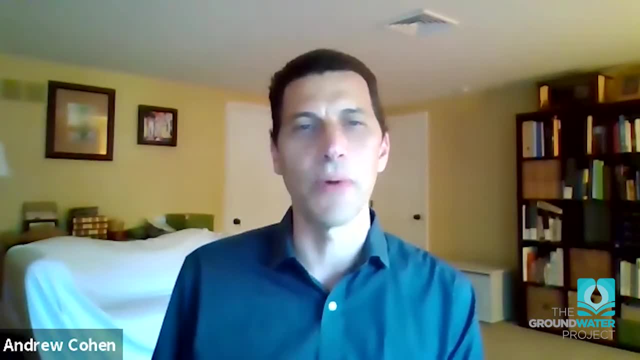 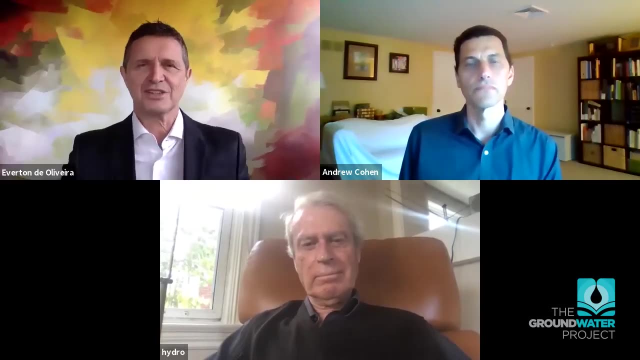 You need to have an intuition as to how it should be, and then the data will help you refine that. Exactly exactly, John. you have something to add about that, Because this is quite important, quite important. People don't see that. 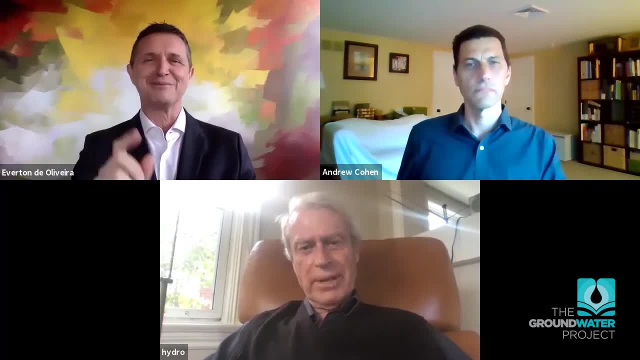 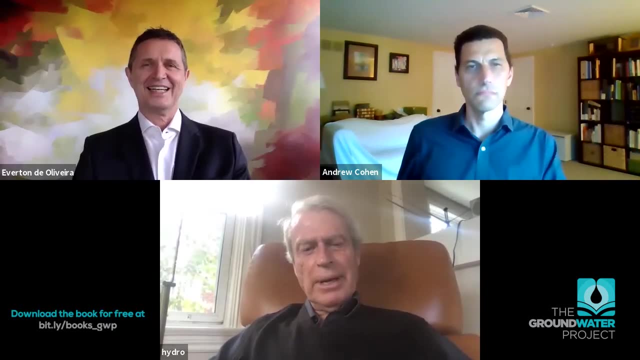 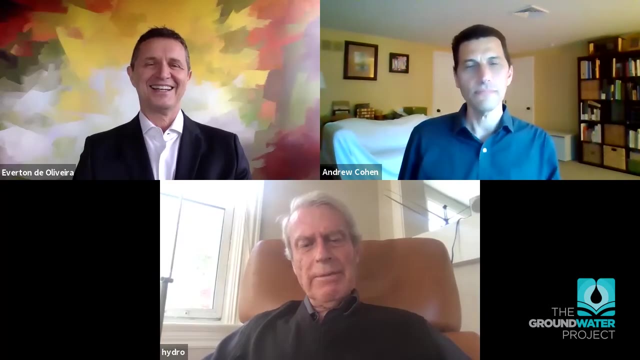 They just think it's like use a triangle and put the dots there and that's enough. no, This book, in a way, is about people having an opportunity to build their hydrogeological IQ- And many of us, when we take our first groundwater course. 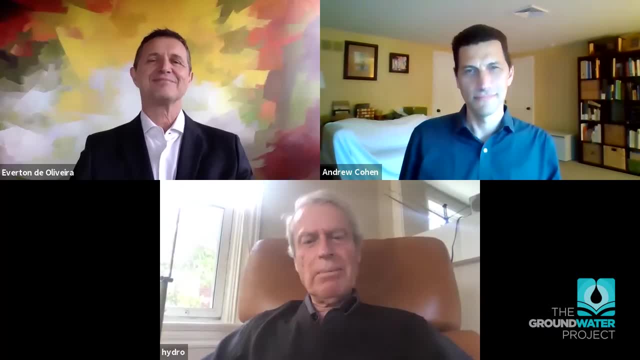 our hydrogeological IQ is very low. I mean, we can be intelligent people, but our hydrogeological IQ is very low, And so it's about basically being able to look at simple numbers: head and K, either one or both. 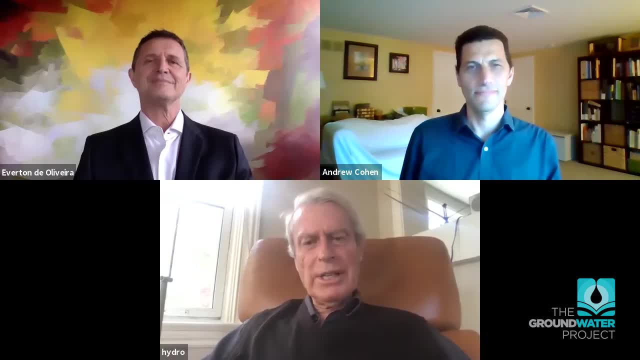 and being able to say something about it, to be able to internalize it and sketch it. In a way, it's about taking information, internalizing it and sketching it. So the sketches- if we call them that- are very simple. 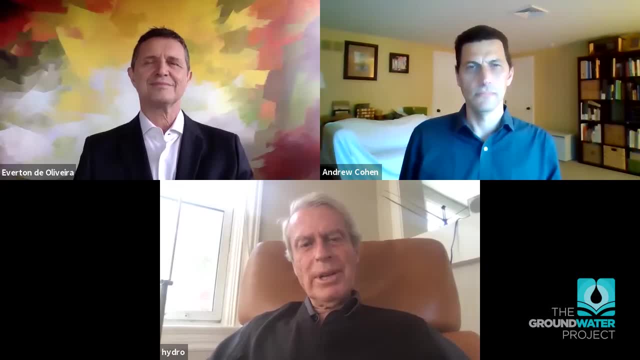 And at the end of the day, we want the reader to take pleasure out of the challenge of sketches. little puzzles converted into sketches And once we got going on this it sort of multiplied. We realized there's so many different ways of expressing it. 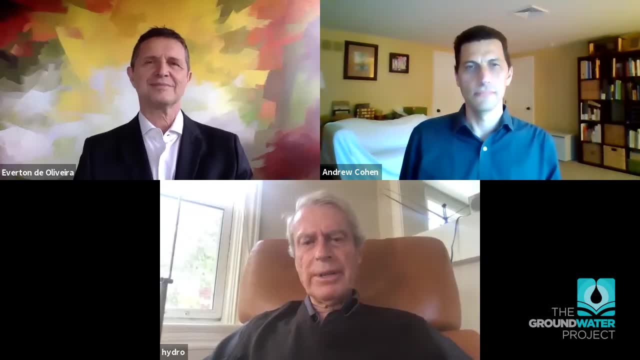 And, if you'll note, some of these figures are very, very carefully designed. Andrew has a particular talent for design And every little arrow and every piece of every figure is thought out to the last detail. And so when you look at it, you say: 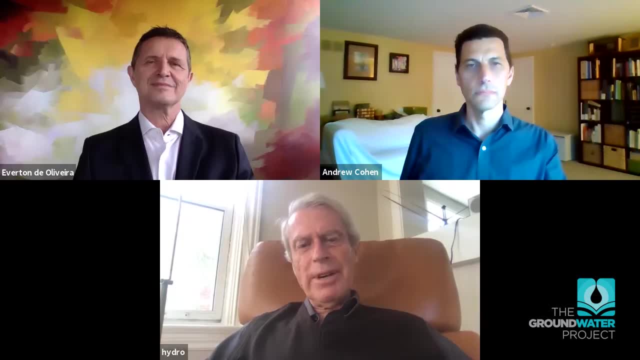 aren't these lovely and simple? Well, they only got lovely and simple by refinement of design And, of course, design. people know that simplicity and clarity are sure Are é of the elegance. yeah, exactly, that's the excellence. that's the excellence when you. 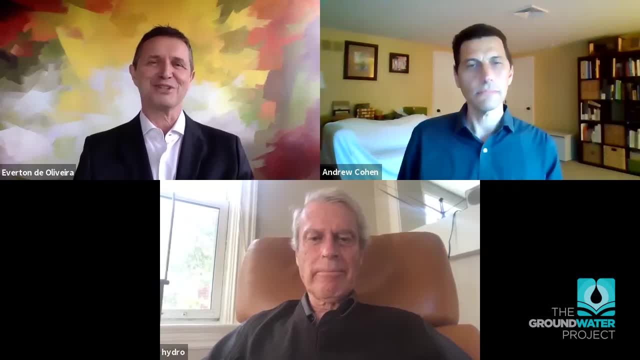 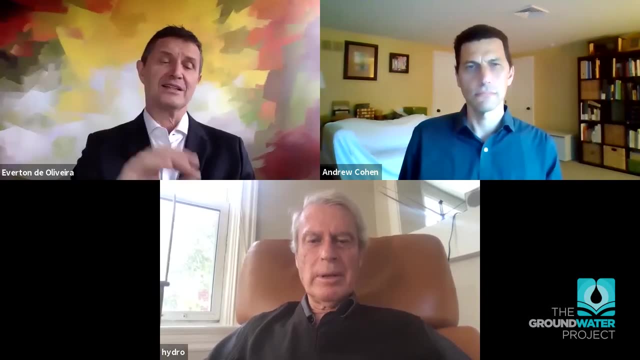 can get it simple, right, this is. this is so difficult to to achieve. actually, i was thinking because we just really released the book, um, uh, groundwater, surface water interaction. and for people who read, who read this book first, uh, this your book first, the books that we're talking about. 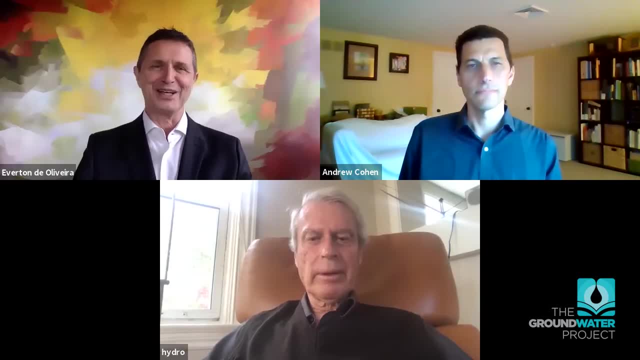 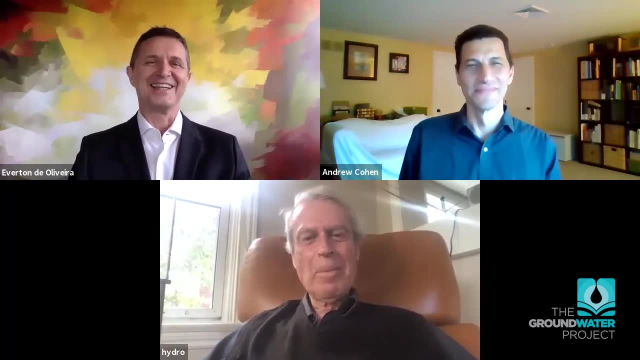 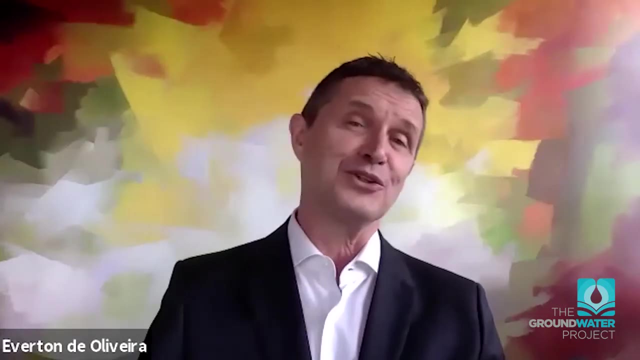 the groundwater- uh, it's a long name, i everybody will say about the darcy's darcy law, darcy's law book that's going to be known as, i think, conceptual and visual understanding of hydraulic head and groundwater flow, if, if we use this first and go to the other book next- oh, this is going to. 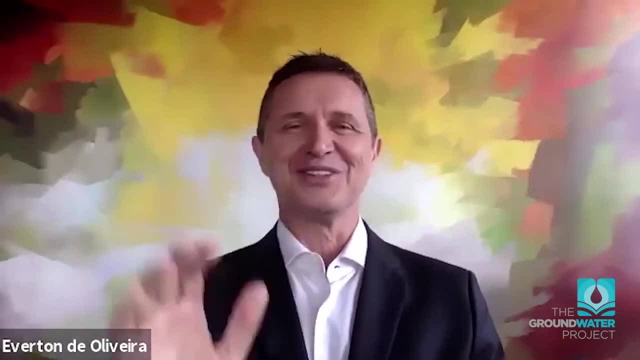 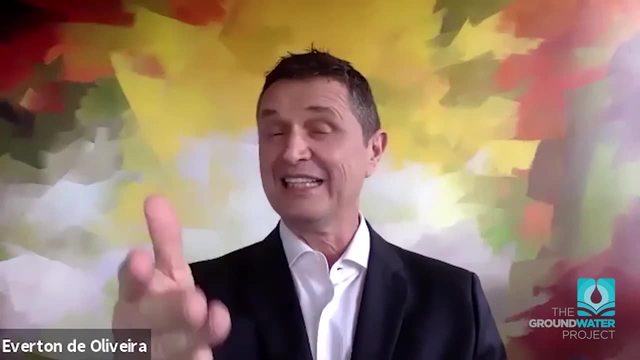 be another word, because it's going to show you you're going to understand things just by looking at it. it's so much easier when you have this book in mind, and that that is a. it's a. actually, for me it's a basis when you go to the field. 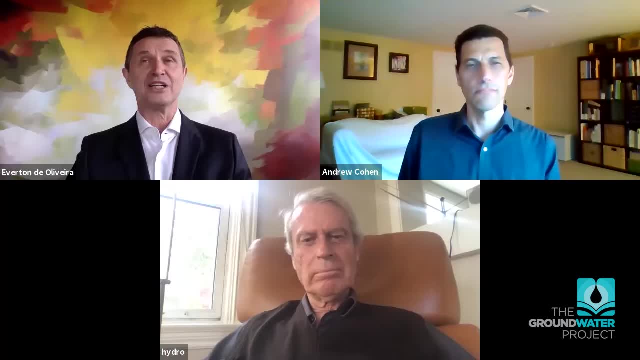 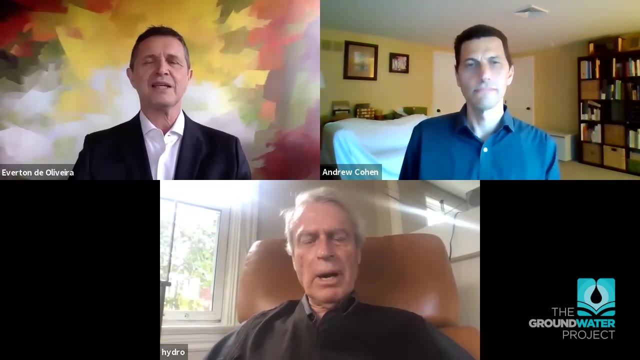 it happens, uh, it helps a lot that you have your, your, your conceptual model, uh done because you have the, the feeling, this, this actually practices your feeling into a great you know, to a much higher level. that's what i think my, my message to the teachers of the world and the teachers. 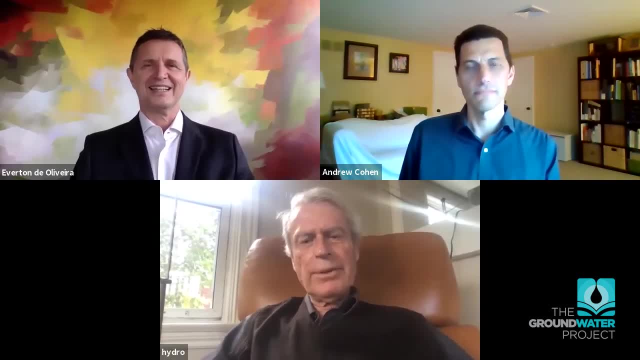 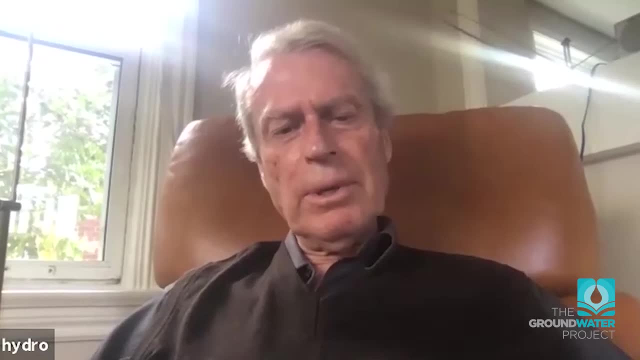 of groundwater, having written the freeze and cherry text that you, you know, was supposed to be so, so good, and it was a good book, but not, not for learning. so this book, then, is for learning, uh, and it's the starting point. um, in essence, it's the starting. 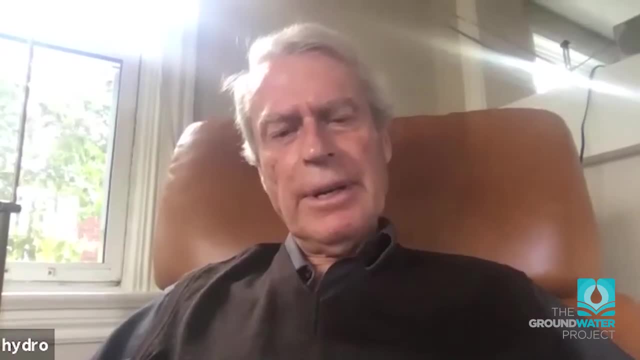 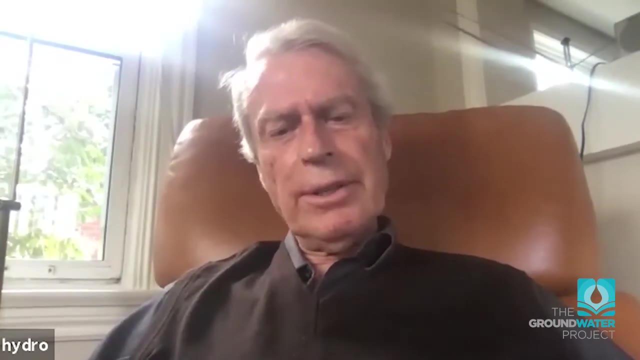 point, and i think the challenge that professors are going to have is is how much of this do they want to try and teach from the book? or are they going to say to their students: study this book for two weeks, and study it for two weeks, and then we'll get the class going? 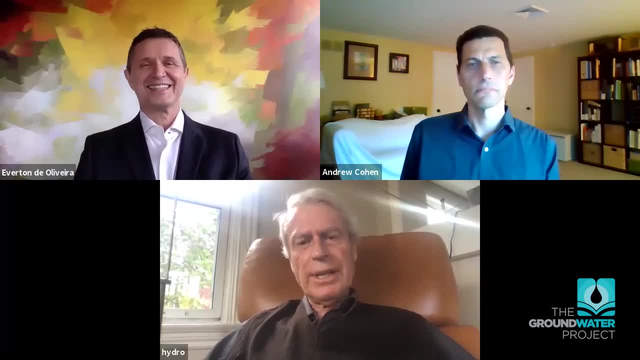 uh, you know, in a way you can just sit and study it and practice. and if you understand all the diagrams, if you understand them and can reproduce them, then you're ready to take the class. and, as i mentioned, i'm always, was always, amazed when i was teaching, how, when i'd move on some things. 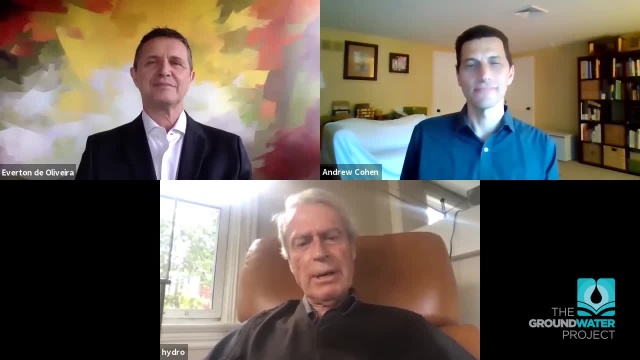 are more complicated. uh, how basically i, i would lose the students. there was something lost there, uh, and i didn't know what, didn't know how to fix it. i lived with it and now, now we have, i believe, a fixed. No, I think so. Actually, this is a very good example of what the groundwater project came. 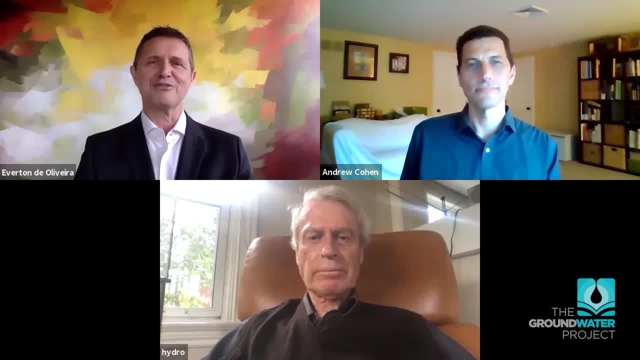 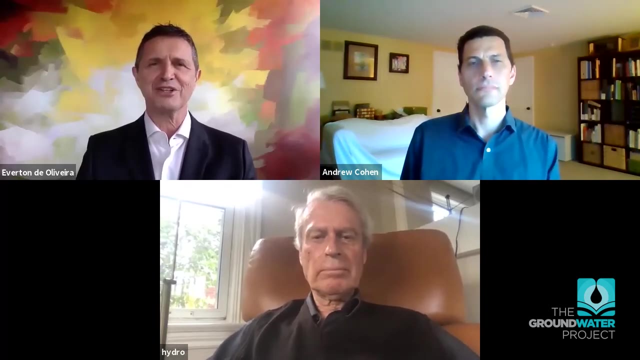 in for right Because we have this very first great example. what do we have right On a single subject that explains everything? I had an example When I was studying to get into university I had this very old professor. He was a mathematician And he has this great book for. 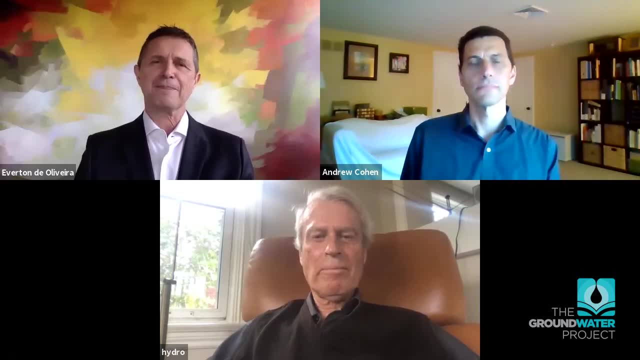 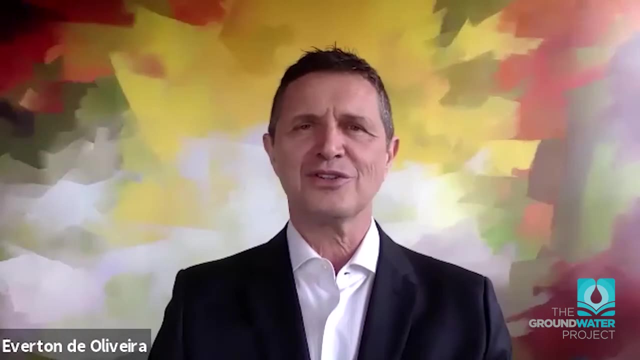 high school And he was a self-taught person. He never went to school at all And he was amazing, So good And usually in his classes. I always remember because he used to go there and he used to explain things in 10 minutes. 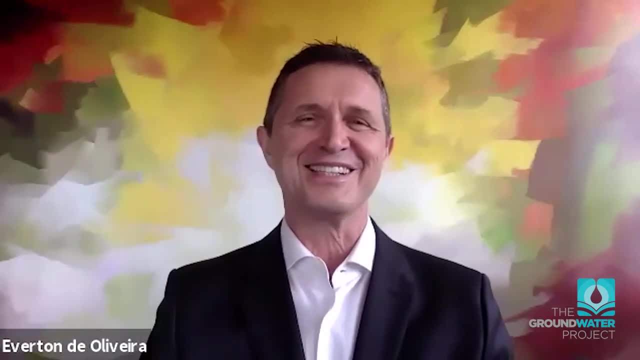 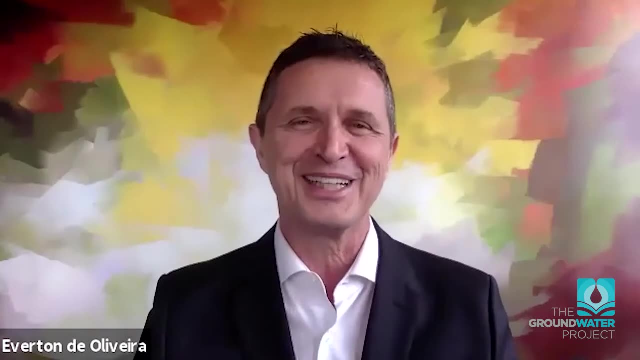 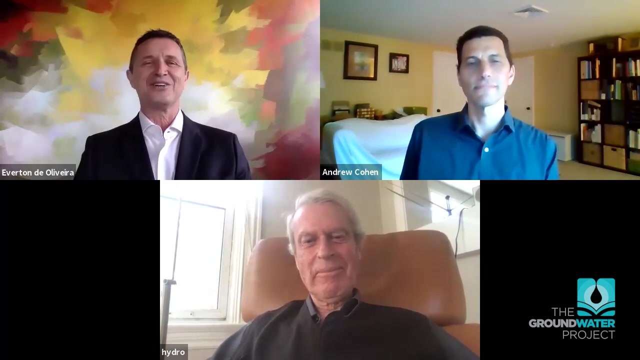 And he goes. it was very you know the essence of things. And then he gives you some exercise And the class was always in a huge silence. Everybody was working, having fun, And I said: how can he do that? right, And so that's exactly what we see. You have a book there. 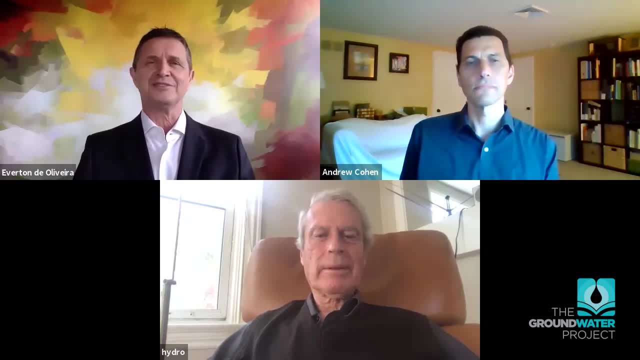 and you have the examples And you can do it on your own. You don't have to read much because you have the simple message up there And then you go and do it. So what do you expect or how and when you expect people should use that At what time? 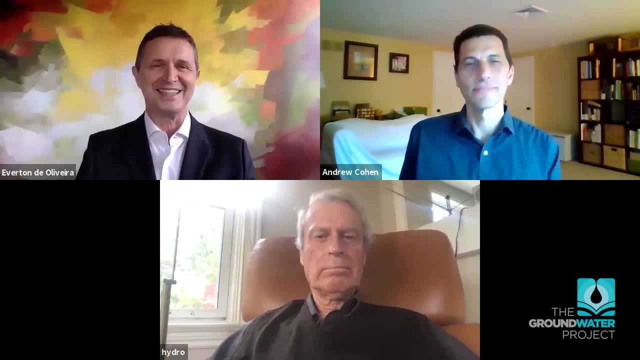 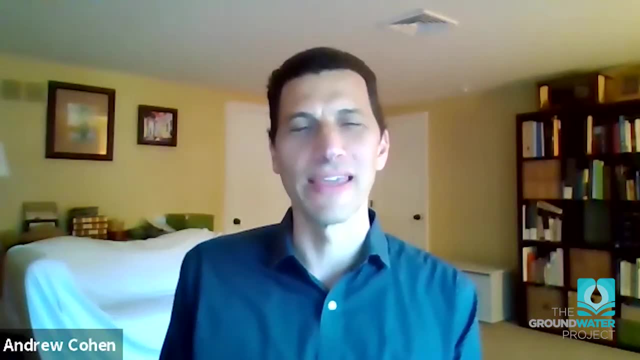 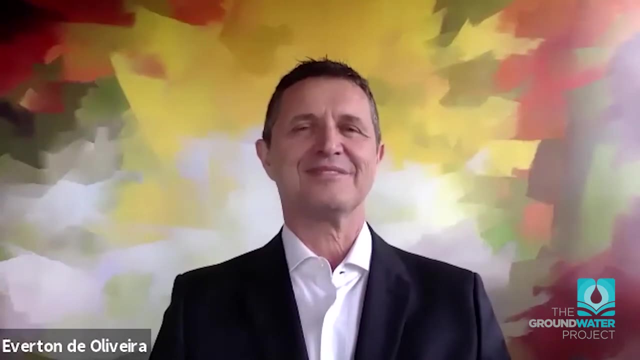 You know later in their career, early at school or any time, What do you think? So this is a book that I think people should look at from the very beginning, because it really just lays down the fundamentals And one thing that I think. 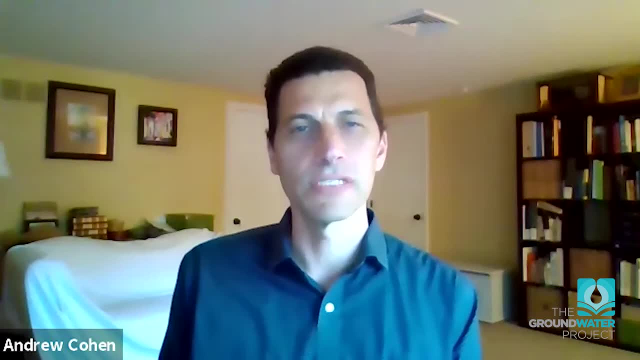 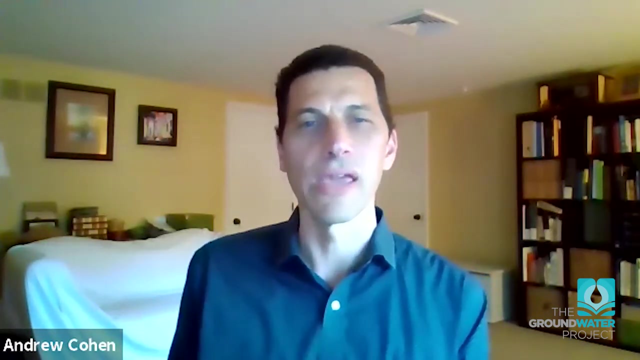 is very helpful. there are some example problems that the student can do And we do provide answers, But we also don't. in addition to providing the correct answer, we explain why the incorrect answers are incorrect from a conceptual perspective. So the student might. 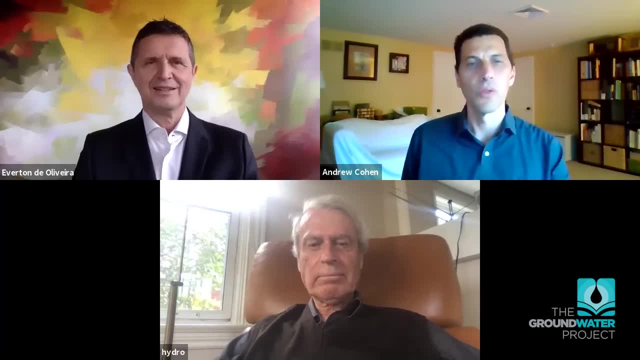 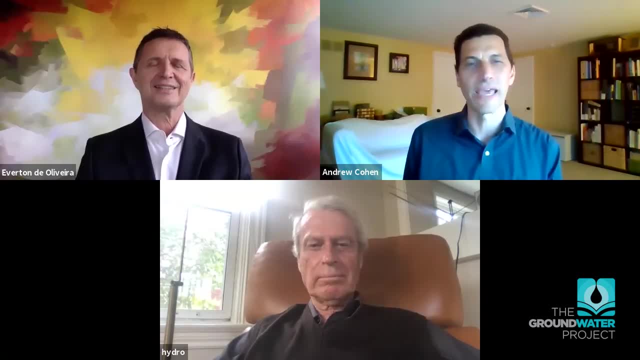 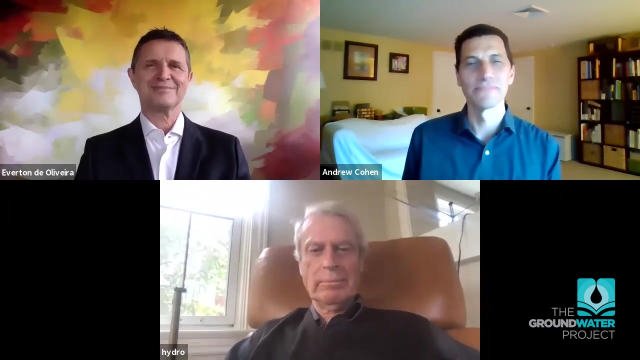 But also the incorrect answers are explained And that provides, I think, a deeper understanding of the essential elements, or it provides a deeper understanding. So there's a lot of learning, that there's a lot of much can be learned by understanding why an answer is not correct. 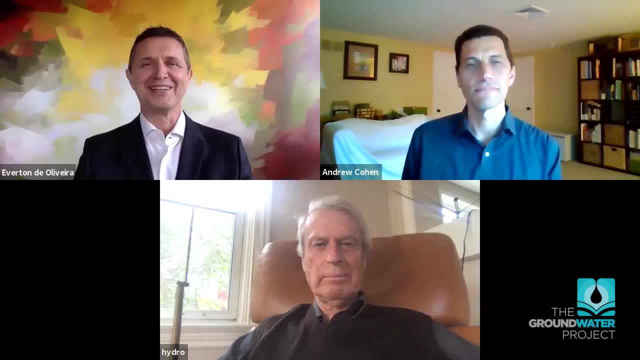 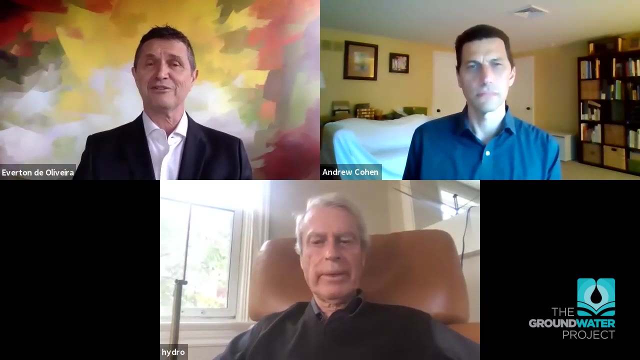 Exactly. Actually, we learn more when we don't do well On a case on the exam, right that you have to redo everything, then you do learn it. That's the idea. So you get the wrong answer and go through it. Actually, just to make sure we don't have only 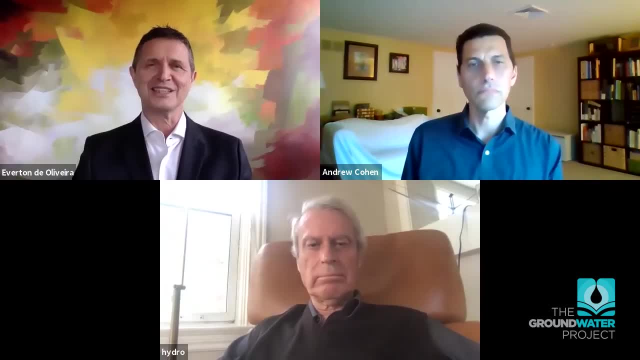 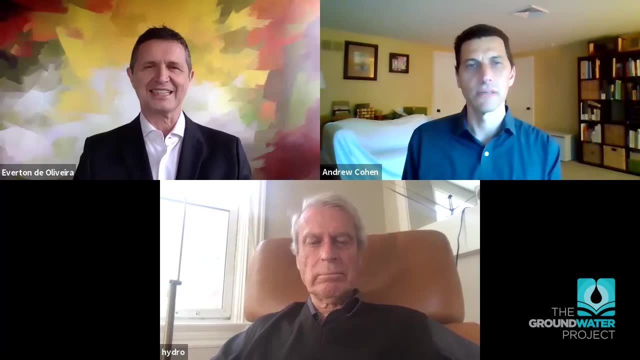 answers. we have solutions in the book, right, We have a whole solution: Tell, explain. That's right, Yeah, that's right. Explanatory solution. Exactly, Exactly, Very good, Very good. I think that one of the challenges then for professors when they use those. 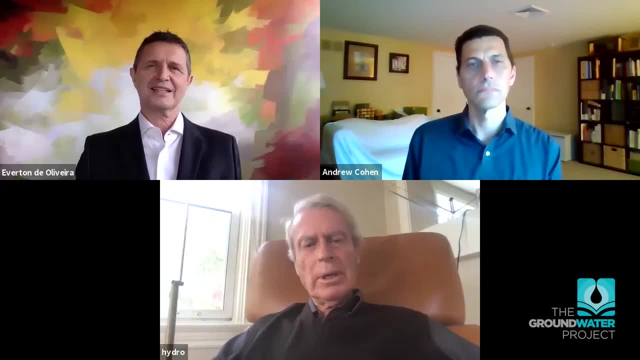 the chapter. it's set up for the student to work the way through it, you know, looking at the problems and then trying to do them and then seeing if they got them right, And then I think the challenge to professors then will be, within this theme, to make up new problems, for which 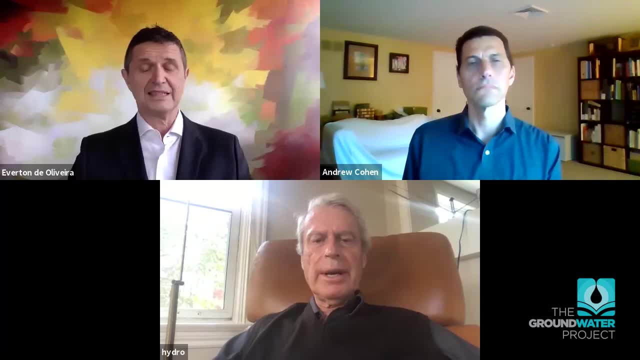 there aren't answers. So what can professors add to the game? Well, they need to make up new problems, And those are challenging, And even the students should be expected to make up new versions of these problems and provide solutions to them. It's like basically a jigsaw puzzle, you know. 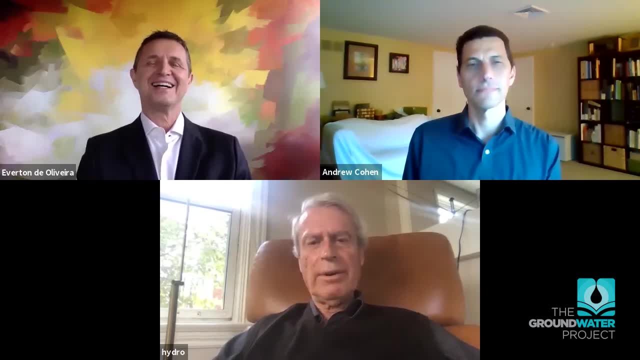 and the manufacturer makes one, and then you can make others and go on forever. And it should be. should be great fun. May I ask you something? What if people suggest new problems for you? would you be able to incorporate into new editions of your book? What do you think? 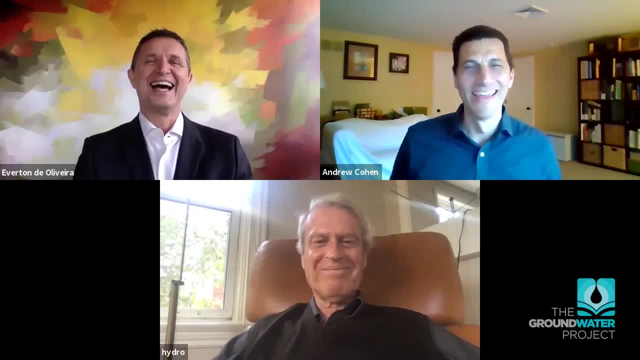 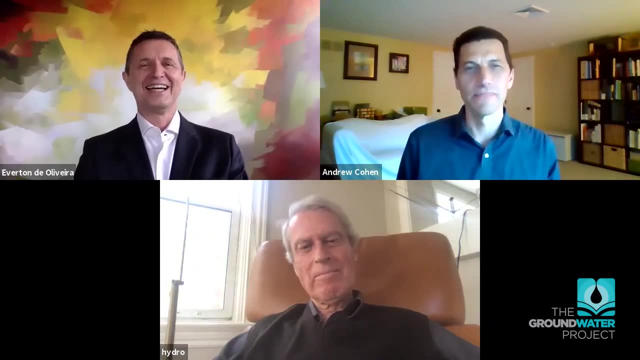 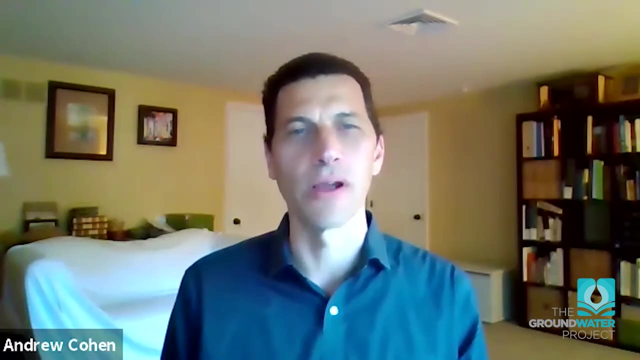 Well, I'll just. you can edit this however you want, But one thing certainly there. So the idea is there. as John said, many different kinds of problems can be formulated. that would be useful for students. that requires them to think in kind. 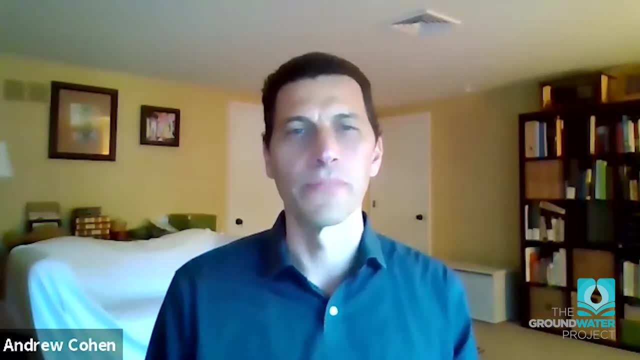 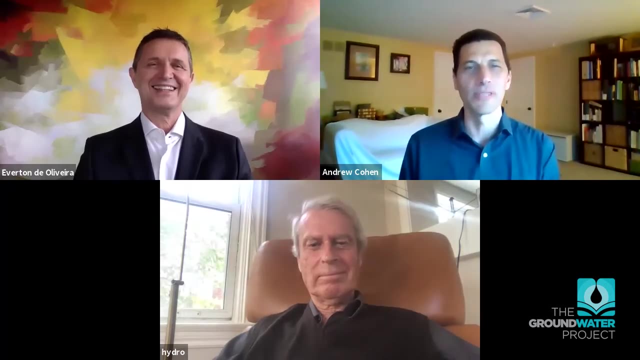 of a conceptual manner or on a on a deeper level. So I'm confident that there are professors around the world who have at least to some extent formulated problems like these in their courses, so they're able to take that situation and write it down and design it in the right way. 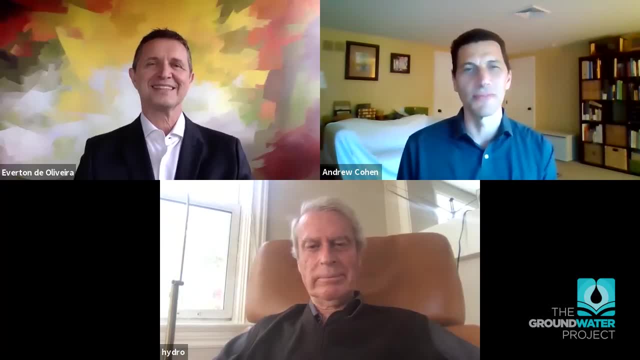 But I think there's a lot of differences between new and existing projects And I think a lot of of the things that are going on, they're going to be the part that is going to be the helpful part of their writing process, And I feel like I have that Mr David is going to say too. 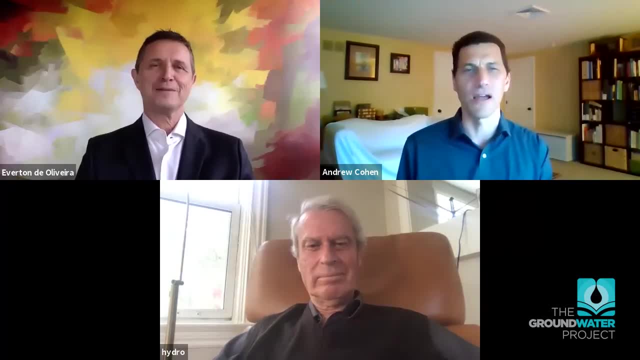 Dr David Donohue, who is with our school here at Berkeley. could you talk a little bit about the work that you're working on, Dr David Donohue MD, Sure, Dr David Donohue MD. And the work that's going on at the University of Colorado? 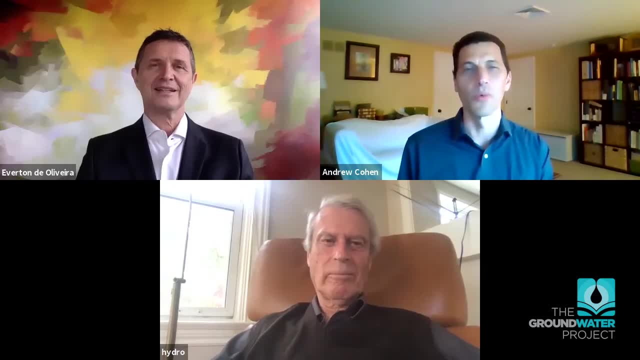 so I'm going to jump right into that. You know one of the things that I do. you know it's the best part of your work in in the real, in the real world, and that's that area, that data interpretation, the development of. 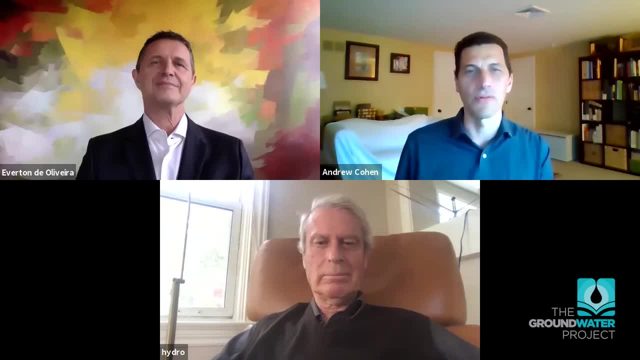 contour lines, which are then used to identify groundwater flow directions. that is something that everyone can benefit in refining their skills, because that most fundamental information can lead people down a rocky road of of making wrong decisions regarding remediation or groundwater exploration or management or identification of aquifers that are sustainable. 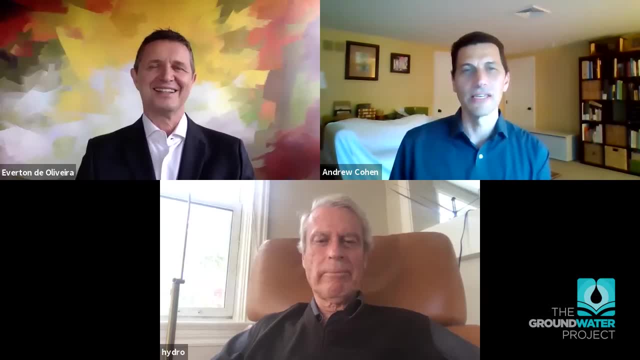 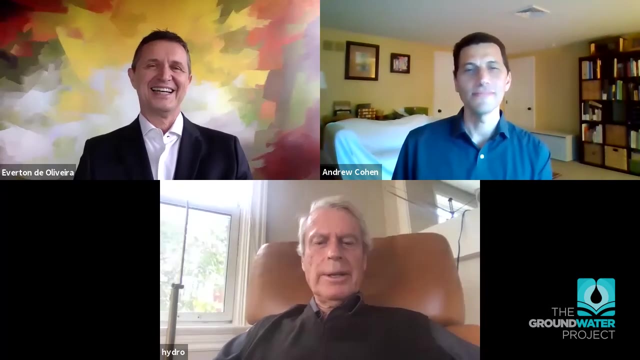 and so forth. really, it's the basis. it's essentially like i said: you don't know anything if you don't know the direction i want to flow. so yeah, yeah, that's true, john, you want to add something? well, the, the, the number of possibilities for little sketch diagrams is is huge, and andrew. 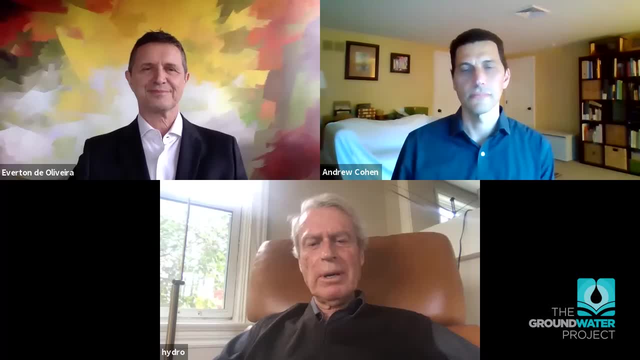 uh, recently ran across an example on the web of a figure where the question is: what's wrong with this figure? and it's just a little head type darcy question and uh one. one could produce dozens of those almost as, uh, you know, universities love to have true or false or whatever, so it lends. 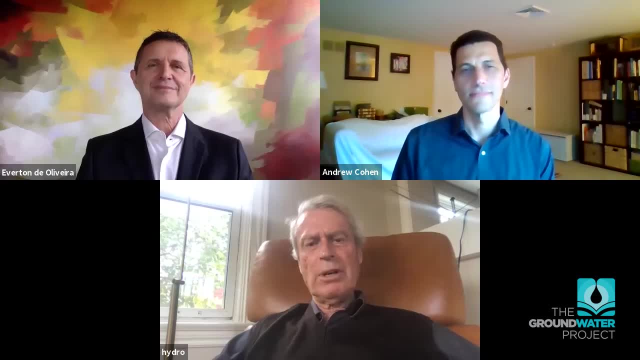 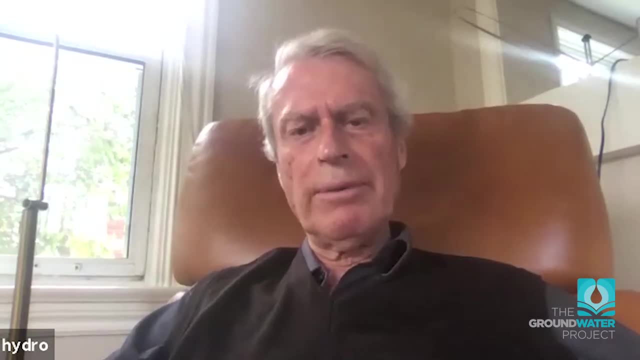 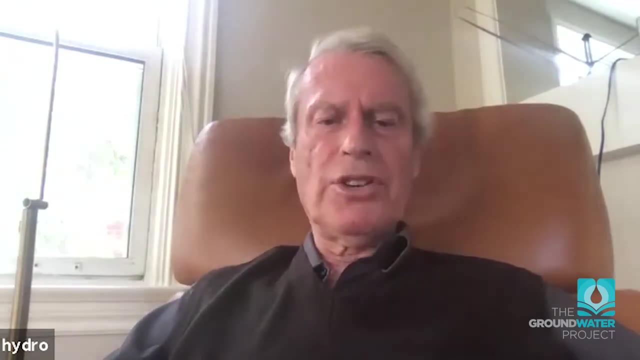 itself. then to all sorts of ways of testing one's knowledge. um, you know, very straightforward, okay, what's the answer? can you do with a four-point scale, right or wrong? you know how to do it with the right or wrong. um, so i think we we've opened up here um a methodology and, as andrew was saying, that, 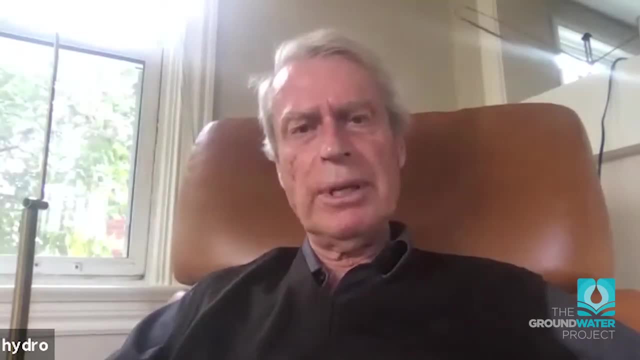 people from all over the world, hopefully, will contribute their contributions to it and this could be a one of the the many wonderful new avenues that the groundwater project is setting loose. and when andrew and i started this, this venture, we really no idea that we were going. 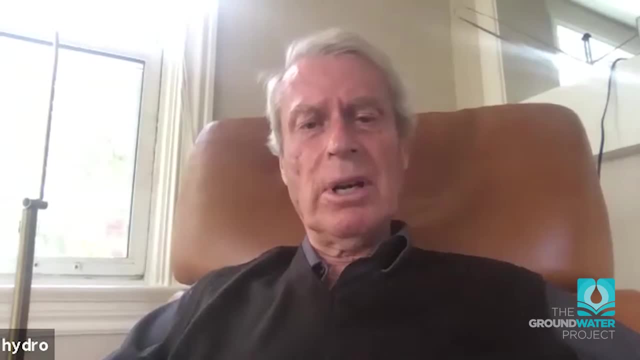 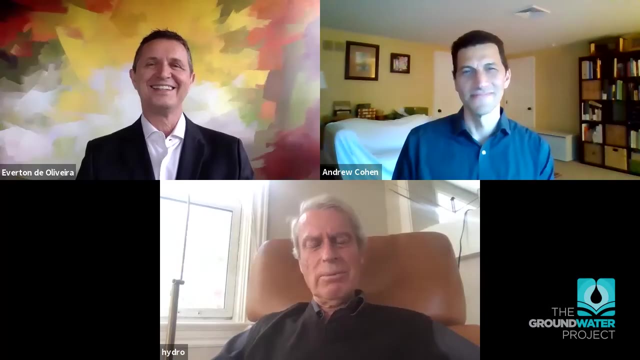 to first of all narrow it, so narrow just darcy's long head, uh. and we had no idea then, in fact, as, as we had to say, stop, i don't. is it for figure 42, andrew? uh, every day or two we're thinking another figure. okay, well, it had. 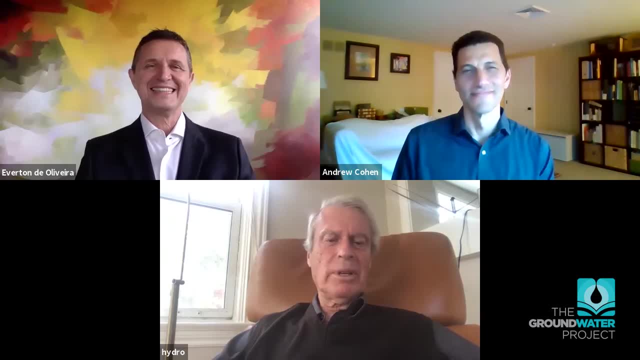 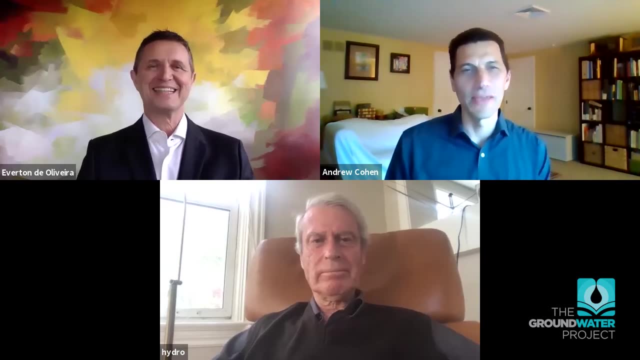 to be stopped because we have to get it published, um, so we've unleashed something, i think, that's creative and exciting and educational and hopefully we'll just see it bloom. yeah, i can it. what it was hard. it was hard to stop creating all those, uh, more figures and 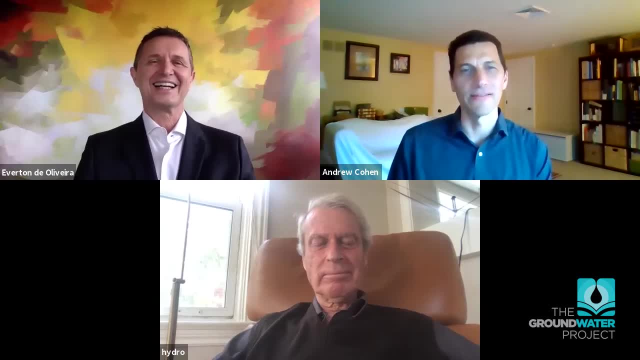 and example problems that provide some additional insight, but they're very good. well, apart from darcy's law- darcy's law, because this book is, uh, all about that. uh, are there more fine cookies coming from this oven? you have more ideas that we can expect? are you working on something else? 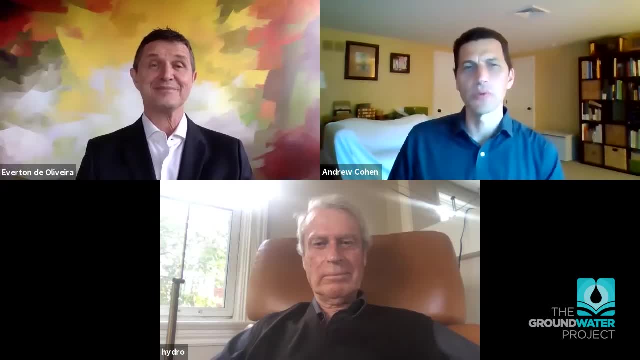 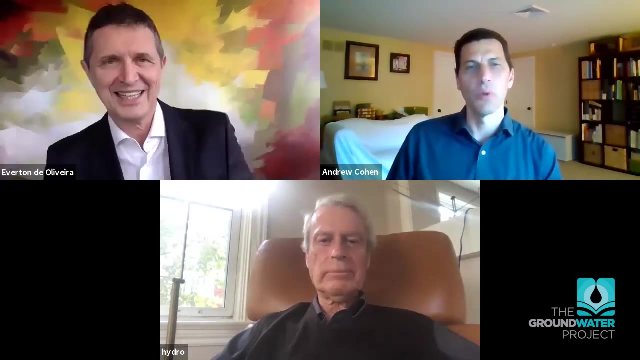 two guys. well, you know, one thing i just want to clarify, because we talk about this being about darcy's law, and i think when people hear that, they do think about the simple. you know, cylinder with a head differential and that's the end of it. but what we've done is we've recognized that, that. 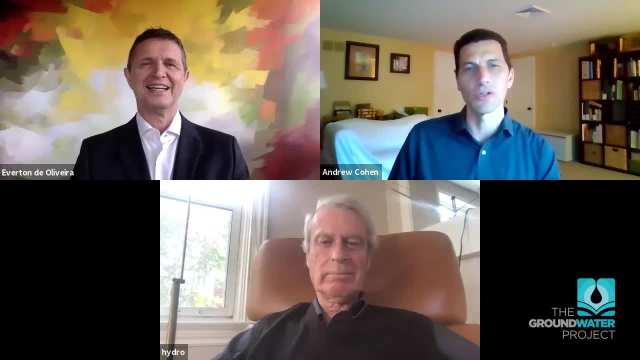 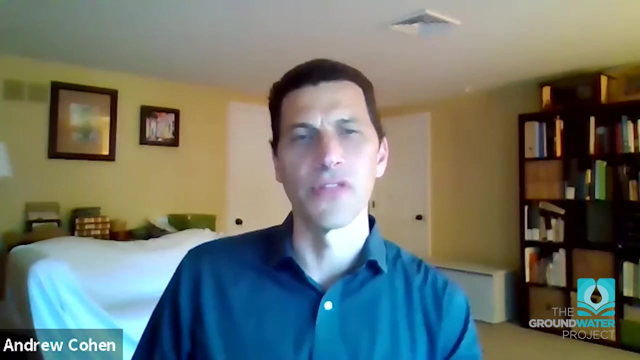 that's also manifested in how we look at contour lines, how hydraulic gradients are a result from various configurations of uh hydraulic conductivity distributions. one thing that we point out, i think, is that's really important. there's a notion that hydraulic gradient drives flow, and that's something you hear. 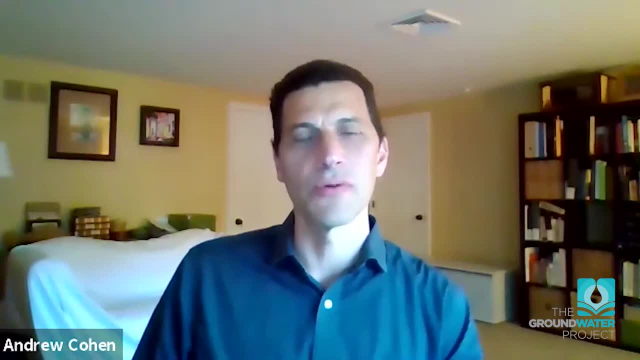 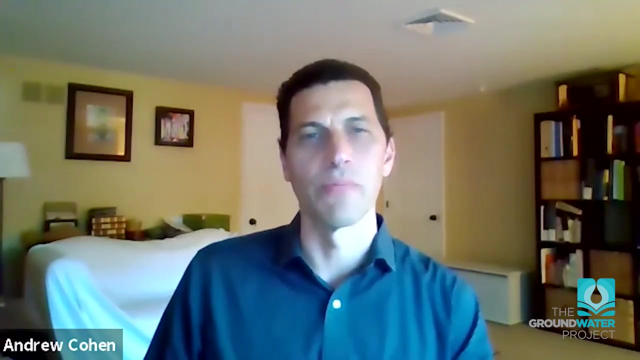 a lot, but i think one thing we try to do is show that hydraulic gradient and the orientations, the resulting orientations of flow, are really a manifestation of the distribution of hydraulic conductivity and your boundary conditions. that is, where are you in relationship to recharge boundaries, discharge boundaries, low permeability layers, so that i think 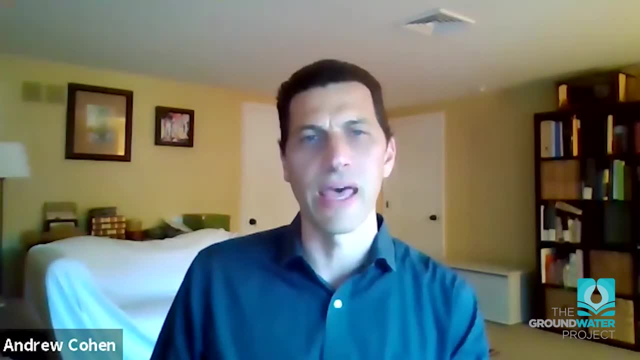 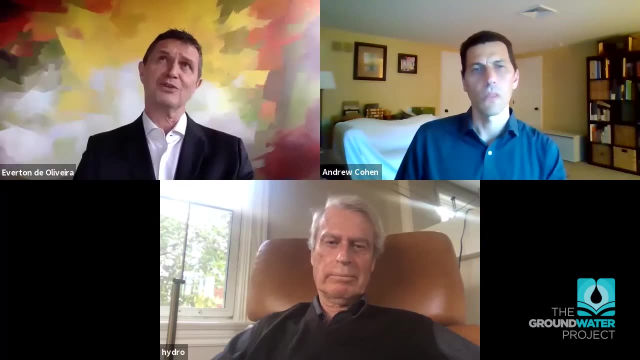 that provides a different perspective that i think will be very informative to people. i agree, for me i have this, this picture, when you, when we, we're working with a conceptual model, because you're always, we're always refining a conceptual model right, and for me, the this book, uh, working with head. 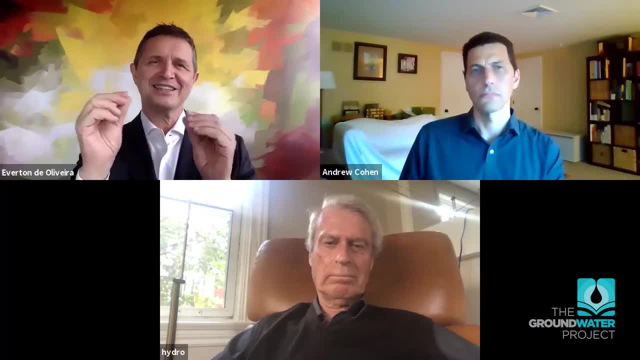 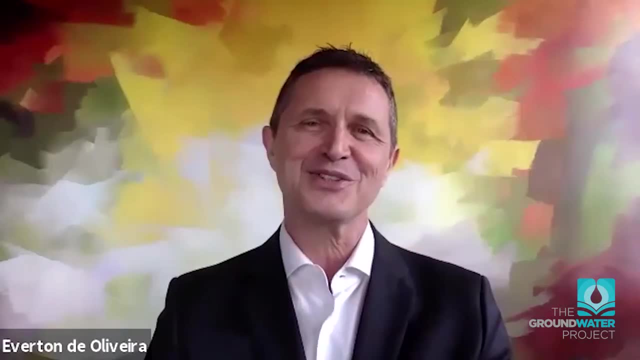 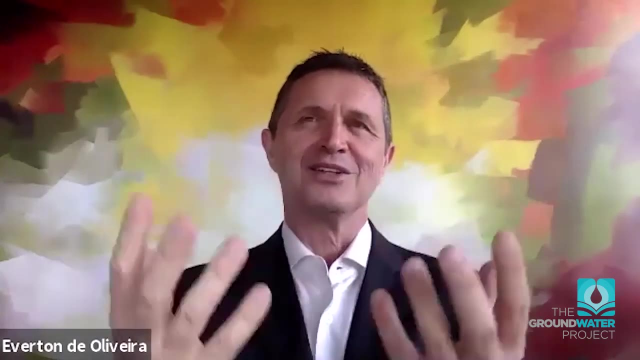 and and k basically, which is actually law. these are the t cells that we can refine your work of art right you? the best you work with these tools, the the best your work of art will be. your conceptual model will be much more you know, representative of the reality if you can work best. 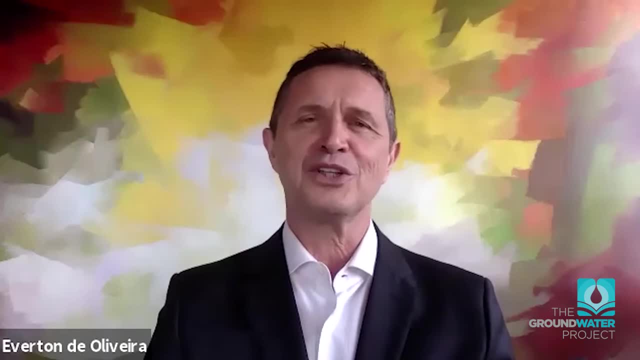 tools and and i i i'm totally with you in that people don't give enough attention to that, to to understand that this is uh all that is, to understand groundwater uh flow properly, which is not, it's not trivial in the real world. it's quite difficult, right. so in this context, everton, 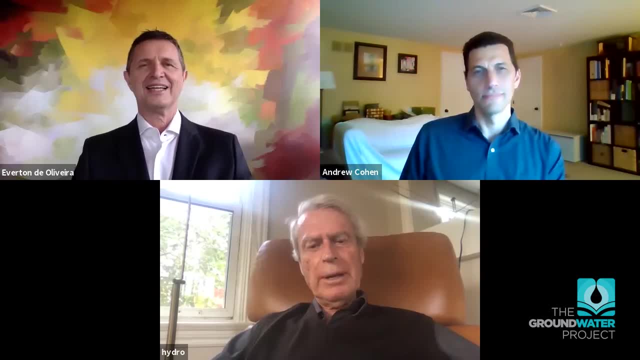 this is very interesting. i suppose another title could have been: you know, conceptual models, conceptual models from nothing more than darcy's law and and head, because all those little sketches are just a conceptual model. yeah, they're for that, and uh, maybe you know when this chapter gets revised, maybe we 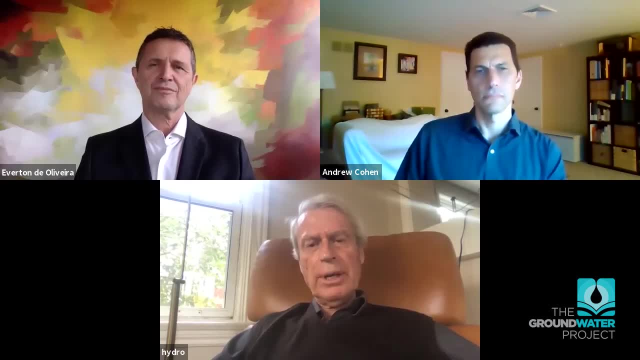 start off using that term more and, as, as andrew pointed out, the chapter actually leads you to understanding what a flow system looks like. yep, uh, what, what, uh, what boundary conditions are like. it sets you up for all sorts of other chapters to come. exactly exactly this is. this is. 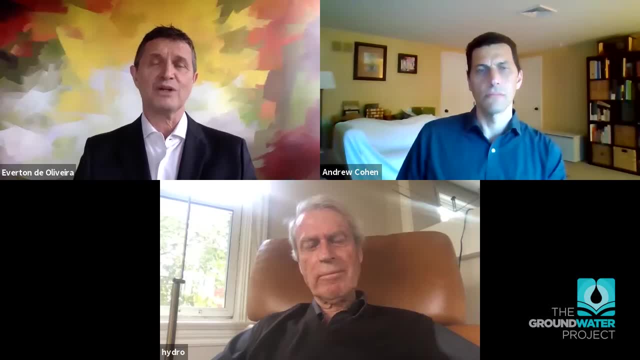 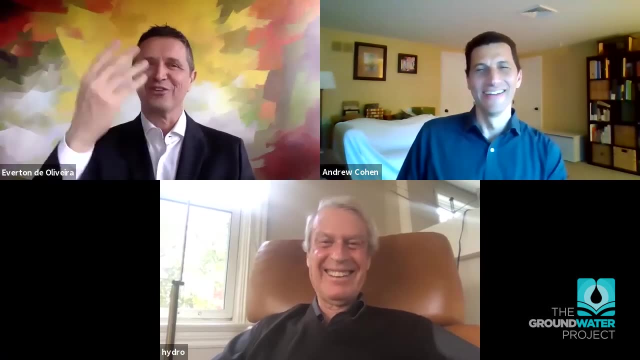 i told you i loved it. that's, that's, that's very good. well, we still have time to change the title. if you want- it's already there- we can re restart the interview with a new title. i the title might be long, but i i think it is. 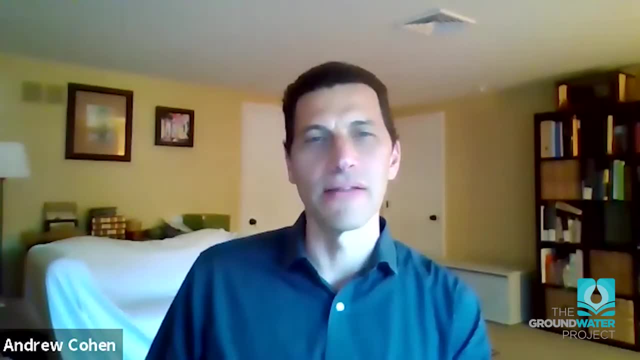 just as an aside, is interesting that, uh, we're not necessarily about subtleties in how you interpret data. what we show, or what the reality is, is that, depending upon how you look at the data, that is, how one interprets water levels, you could come up with very different flow scenarios. 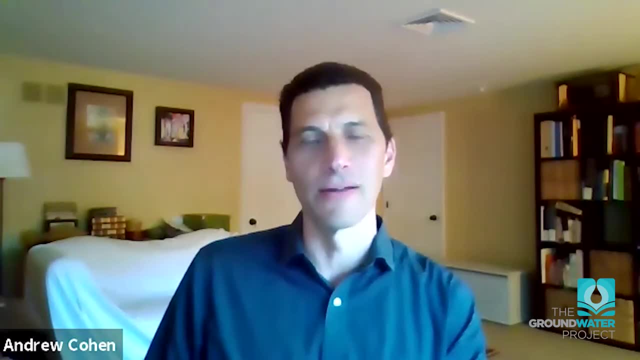 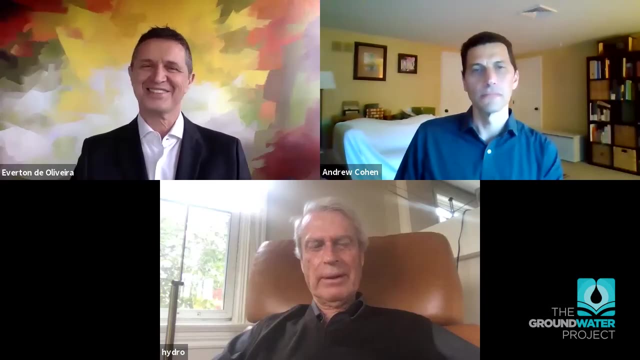 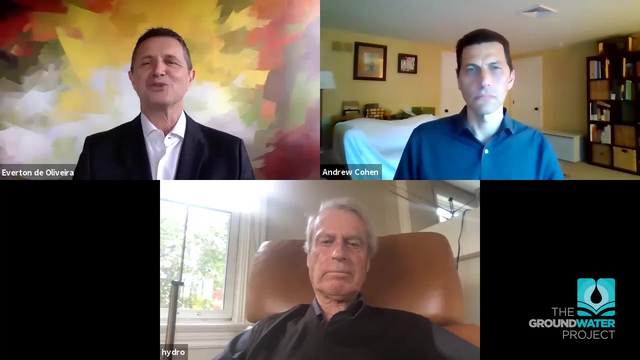 you might think it's a subtle difference, but we're talking about left, right, up or down. I mean it can be actually quite profound. it's quite interesting. it's true. that's true. you like preparing this. nice illustrations from groundwater education. do you have any ideas on how to engage more people like you into the? 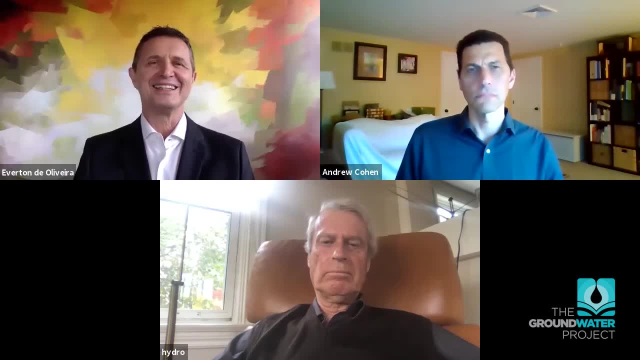 groundwater project to bring in more help. any brainstorm is welcome here, please. well, let's see brainstorming right. so you're correct, I do enjoy. I do enjoy developing these figures and in fact, one possibility is reaching out to other. I'd say earth scientists, geoscientists who have a 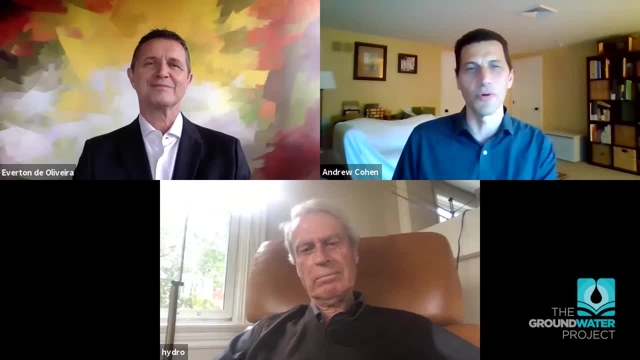 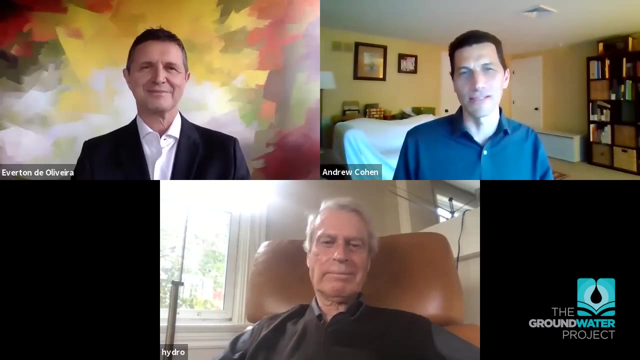 proclivity for for drawing these or making these illustrations, and I can tell you that the people who make the good illustrations really do. it provides a lot of satisfaction for them, so I think they'd be eager to help. I've already reached out to someone else that I know is really quite talented in this area, and she and the 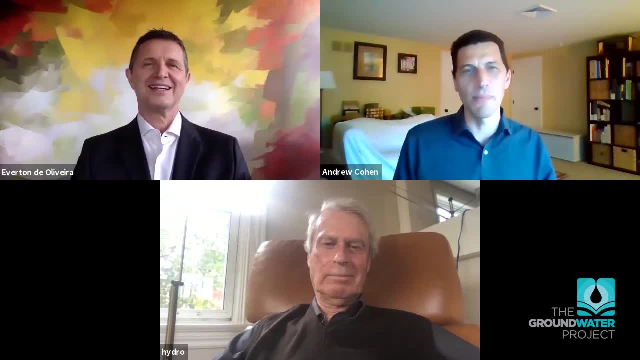 other folks have done it and I've been at the top in the field because I've done a lot of 6th grade- I think I've done about 500 of them- and I've been interested in the software field because I haven't had the time to think about. 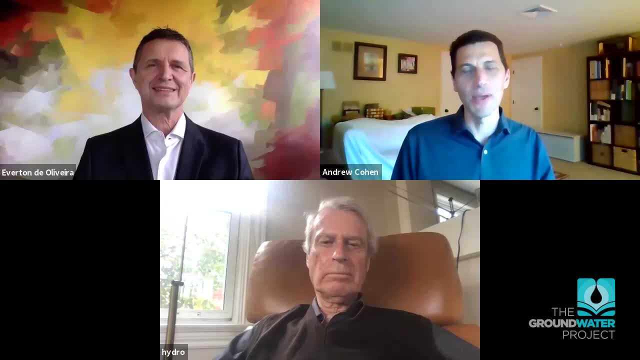 how you're going to be out there and how you're going to be able to make this work in a number of different ways. so thank you, John C. really a big recommendation on the. the next, we've got a question. we've got from a commentator. that is a lot of questions that came in here and I do want 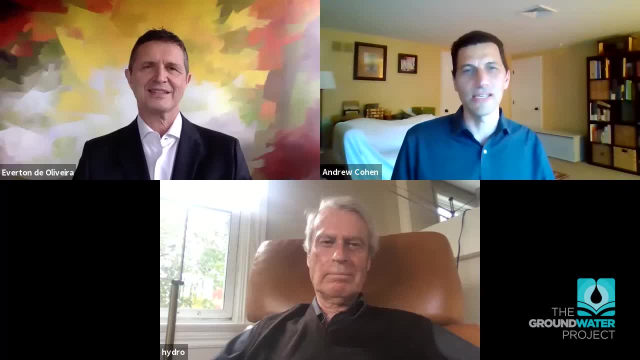 to hear your opinions. please go ahead, John C. And there are many different ways. you'll see in the literature on the internet just even simple cross-sections of how they're presented. So one thing I was thinking is actually to pull together a collection of figures from 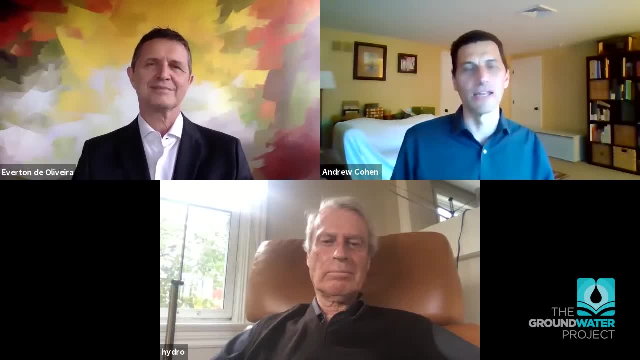 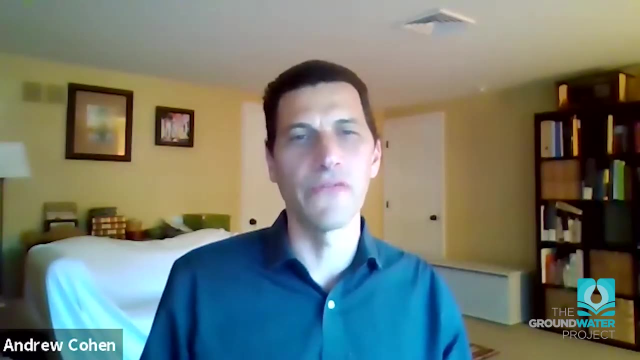 the literature of the same kind of drawing and to distribute that or have some kind of polling to find out which figure is most compelling to students. There's some element to figures that hits home or really conveys a message. It's different. maybe it's a little bit different for different people, but I do believe that. 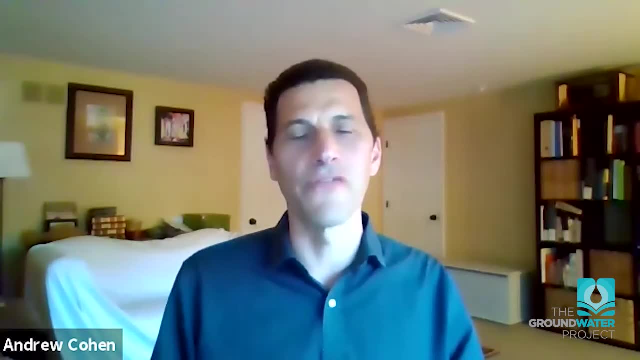 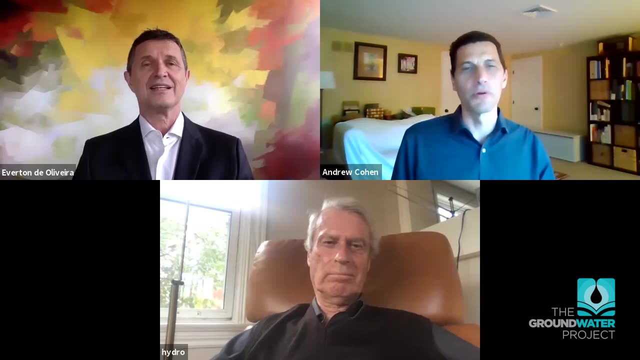 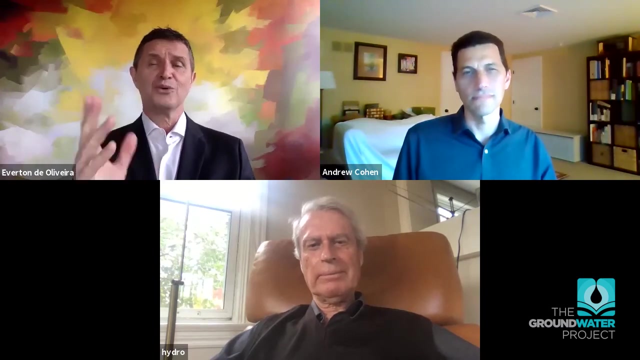 there's some commonalities. It'd be interesting to actually find out what those are, And I think something like the Groundwater Project, some kind of polling mechanism, would be interesting. That's a good idea. that's a good idea. I think we could shore up this idea and see how we can develop. 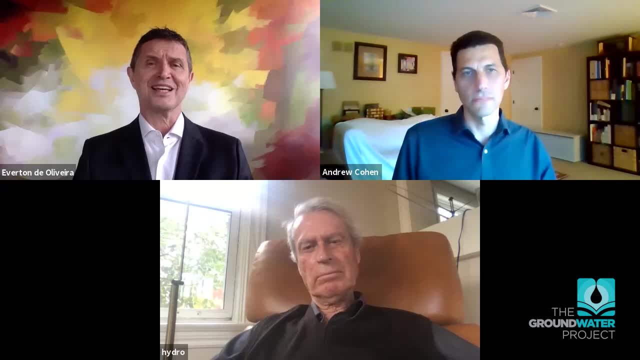 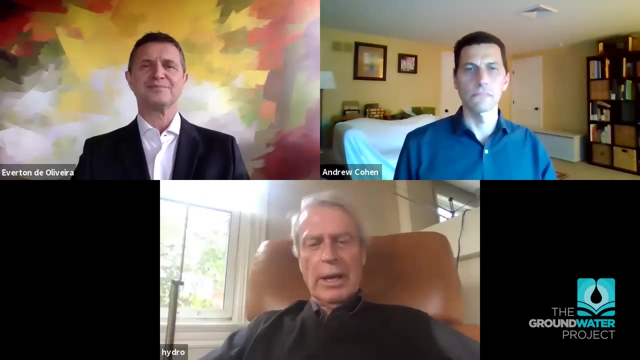 We have a marketing team. they have lots of great ideas on how to engage people and checking things, So I like that idea. Let's see if we can put that into practice. I could ask Andrew a question. These beautiful figures at the end of the day are beautiful. 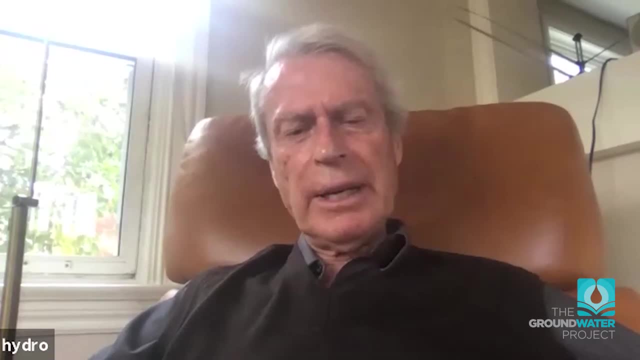 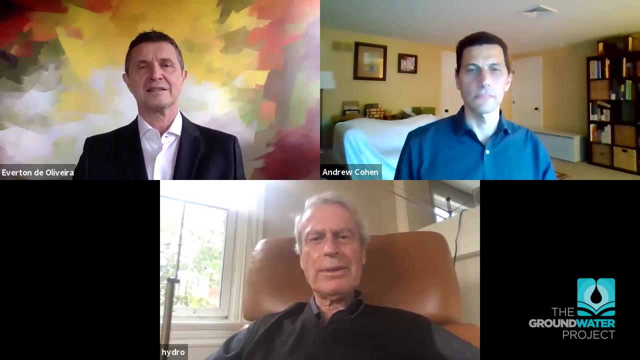 Because, Because of their accuracy of thinking and simplicity and elegance. So, Andrew, how long would it take you to do one of those figures in hours? You probably don't want to think about it because it took so long. Well, I think part of the length came from all of the adjustments to the actual document. 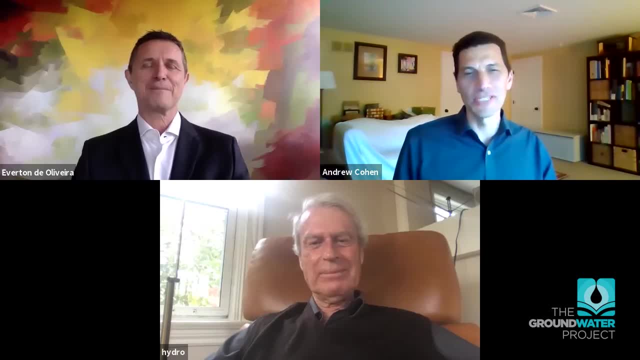 and what material we decided on covering. But I can tell you that the figures themselves took minutes really to draw, to sketch out on. you know, architecturally It was the migrating that over to something like I wound up using PowerPoint might not. 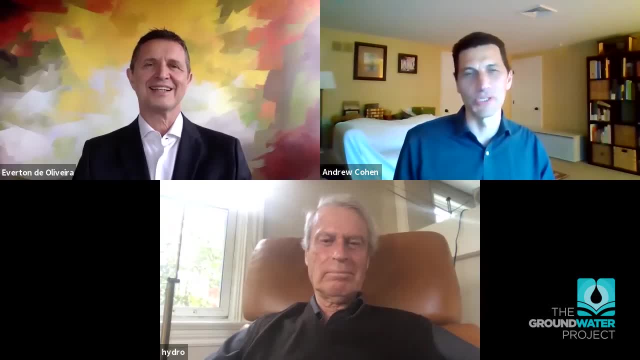 be the most effective way, but I know a lot of tips and tricks and things like that And it's a problem. when you have, when you really like precision and you like things that are beautiful, you can wind up spending a lot of time on the simplest, simplest figure. 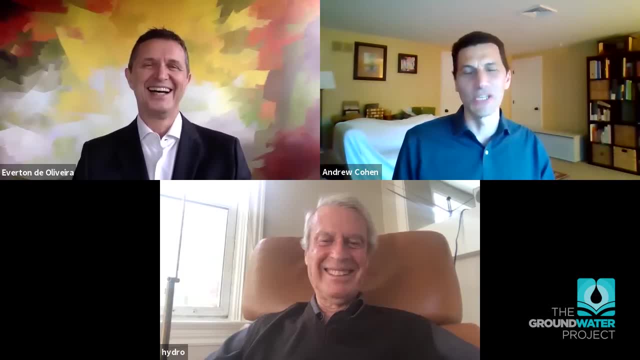 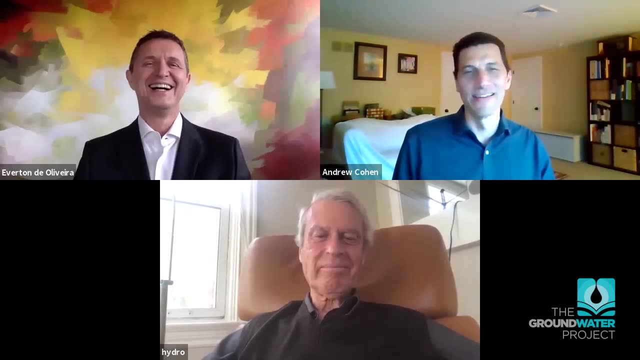 And so you can kind of get addicted to it, And I sometimes need to step back, because there's always room for improvement. And you draft it one time and two weeks later you look at it, you see that the water level symbol is, you know, a micron off of the water surface. 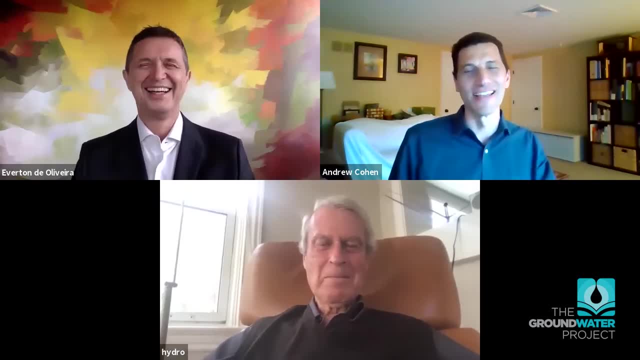 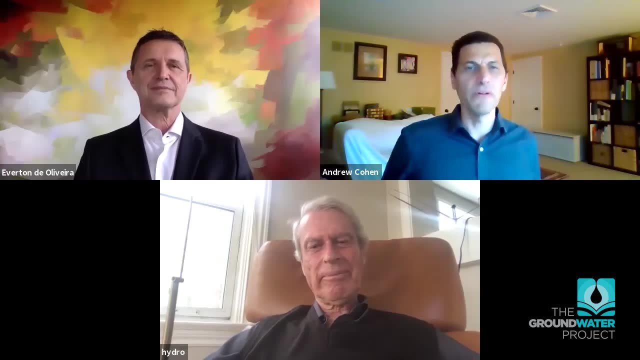 So you spend a half an hour fixing that you know things like this. But actually, John, I think that's important for people to know Simple figures, or you might call them that. they're, they're very, they're very compelling. 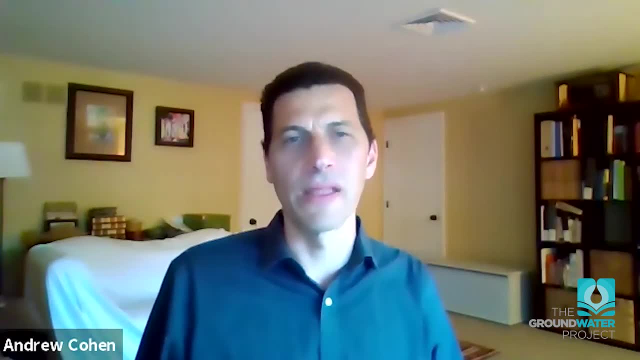 they're elegant. It doesn't mean that they need to take a long time. It's really these kind of sketches. they're just formalized in this book But they're just neat. they're neater publishable representations of something just drawn with. 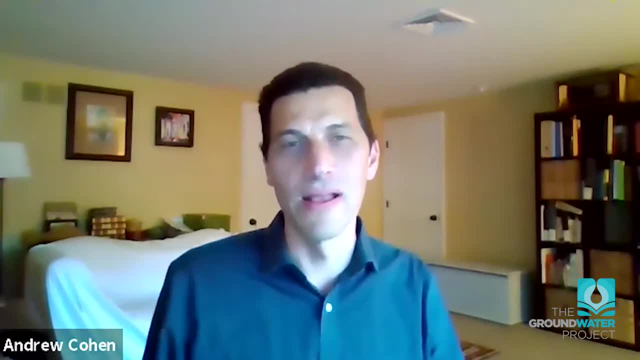 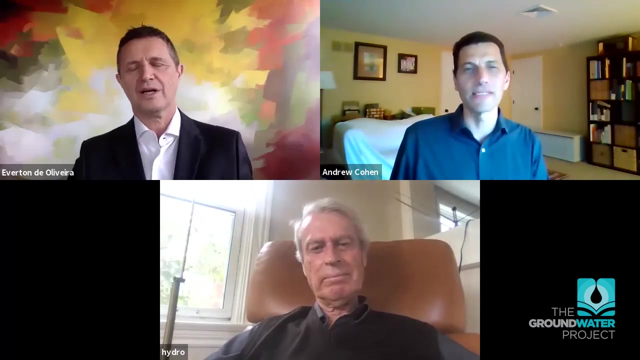 a pencil on graph paper or not even graph paper, And I think that's something that the student might keep in mind- is that these are problems that you really could sketch very quickly And in fact, it would be nice. maybe one goal is for the people that are learning or trying. 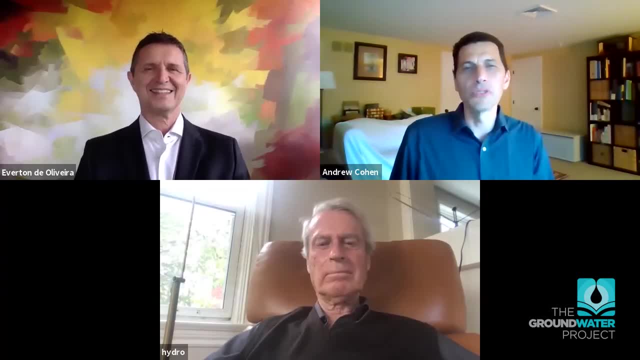 to understand this is to get to a place where, if you posed a problem to them, they would simply they would be able to sketch it out. And that's where that conceptual- you know that coupled conceptual and visual- Understanding comes into play. it's like, okay, do I, can I conceptualize what the issue? 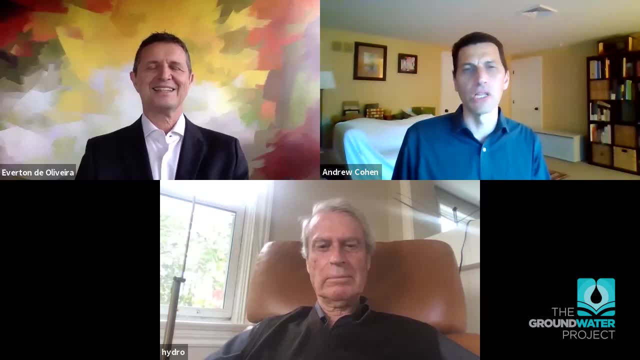 is. And then can I? can I imagine what it looks like? Can I imagine what the corresponding shape of the contour lines need to look like and be able to sketch it? That's really the foundation of every project I've ever worked on. 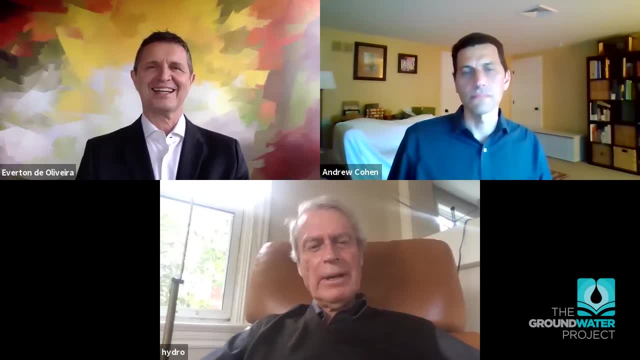 Late, late in my teaching career, before I gave up, I got to the point. I got to the point of of having many exam questions where the question was a paragraph. Imagine a situation where you have two layers and a bunch of wells, and here are the head. 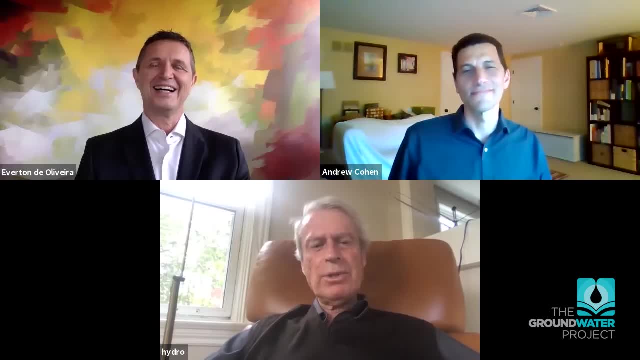 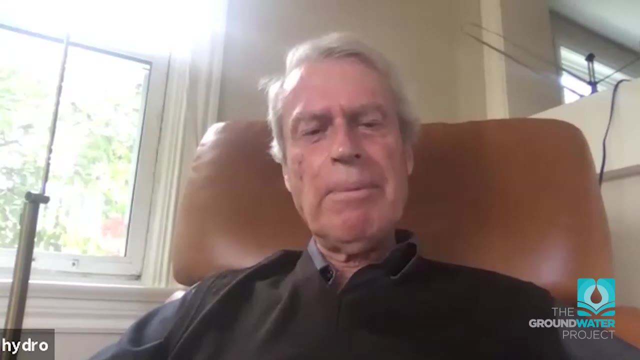 data head numbers, And then I would ask the students to express that in a, in a carefully labeled sketch figure, And what I found disappointingly in many cases is that is that now they would give me a paragraph back or they would scratch something off that I couldn't understand. 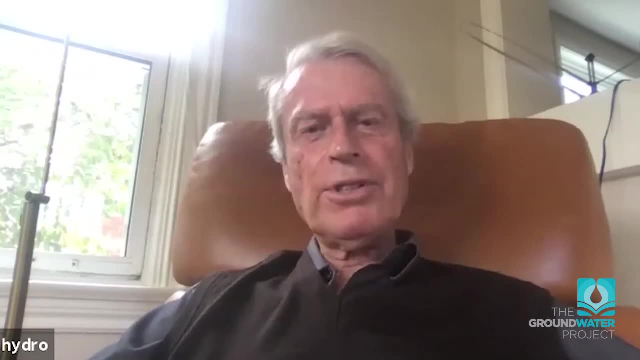 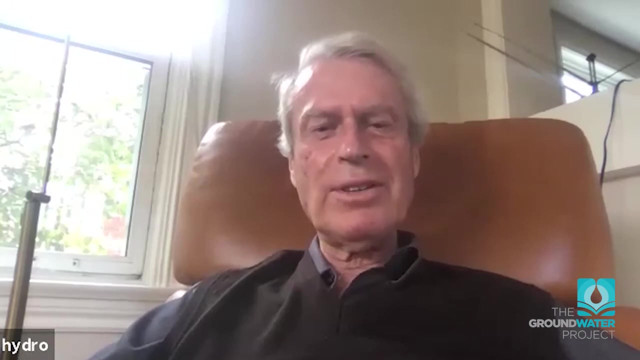 Um, and then eventually, in order to force them to sketch, I would say, no marks are given for words or equations, And that caused great, great psychological strain and terror. you know it's, it's not taught, It's the essence of hydrogeology and it's not taught. 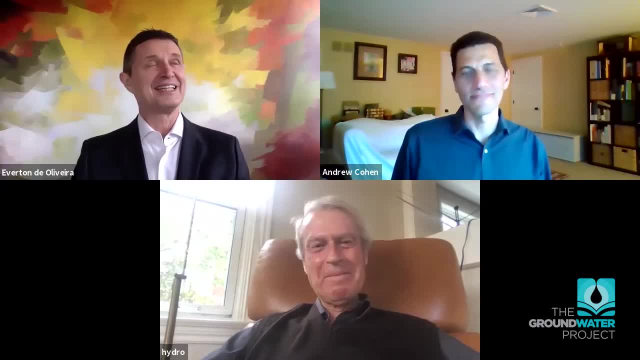 Well, but coming up with that, well, the actually, uh, making the final sketch or a final drawing is not, is not all. Yeah, That's all the point. The point is is having the, the, the, the clear situation in mind, right. 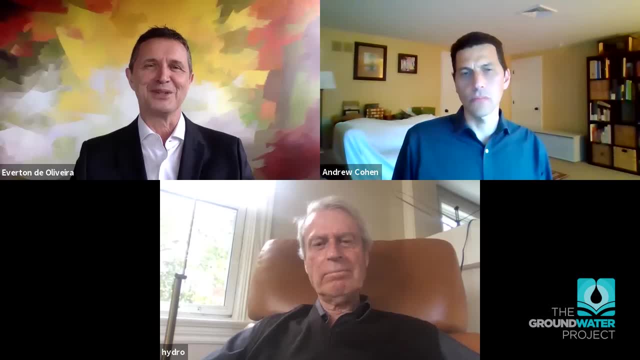 Then you you can, you can put into the paper what you're thinking. If you don't think properly, the you know the sketch will never be good. Right, Because it has to be clear on your mind. So when you know a lot about the groundwater, you can make some good drawings because you 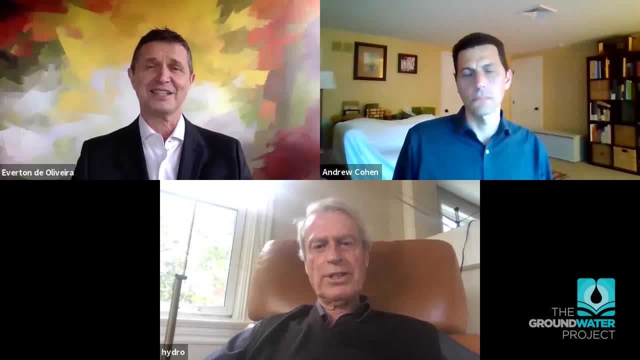 have it in your head. This is not. this is not easy. That's the goal. That's the goal of this book. Yeah, Guys, our talk is very good here, but we, we, we, we need to to get to to an end. 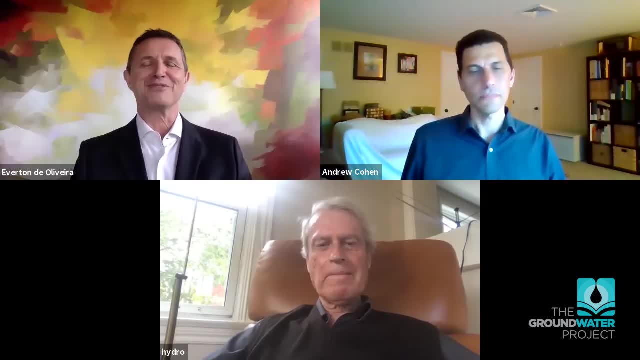 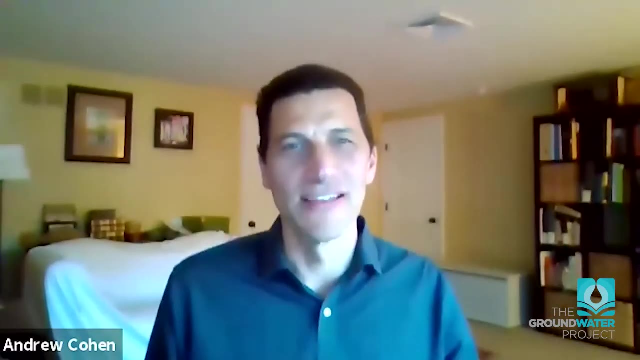 Please would you make your final stand statements for those who are still in doubt if they should download this book, please, Anyone, Sure, Sure, Okay. So I think the reader will. well, the first part is that it's free to use and you'll find. 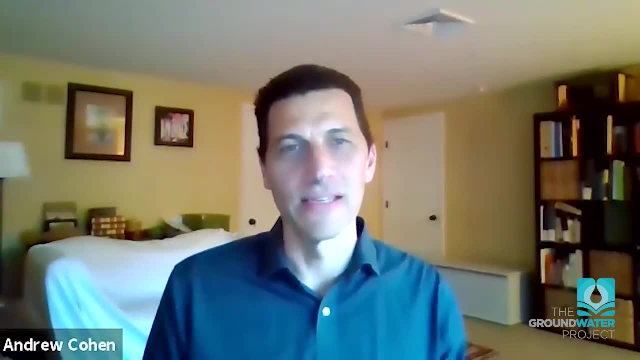 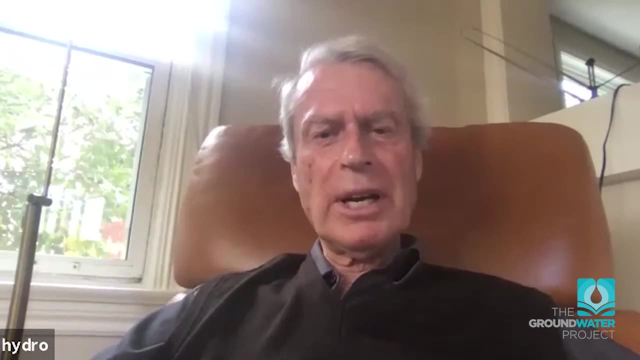 I think that it's quite fun. In fact, this book is a starting point for learning about groundwater science. You cannot start from a more basic level than this, And it works your way up to to quite an advanced level of thinking by looking at pictures. 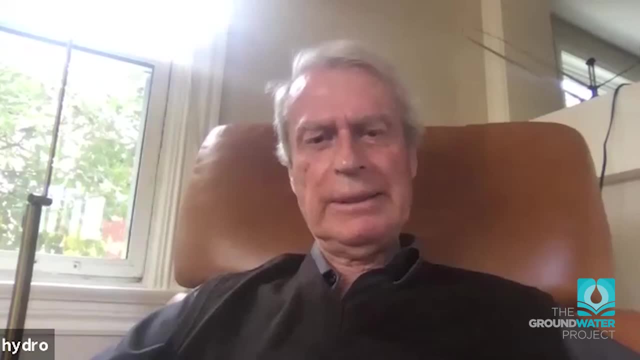 by doing the problems and by pondering. Um. so it. of all the books in the Groundwater Project, If you want to start learning groundwater, this is the one, and it could be done in high school. Um, it's, it's a book for anyone. 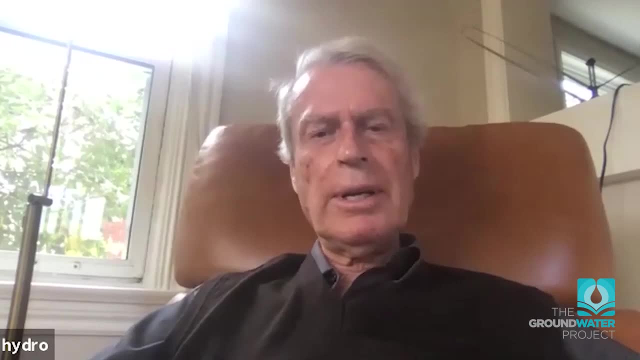 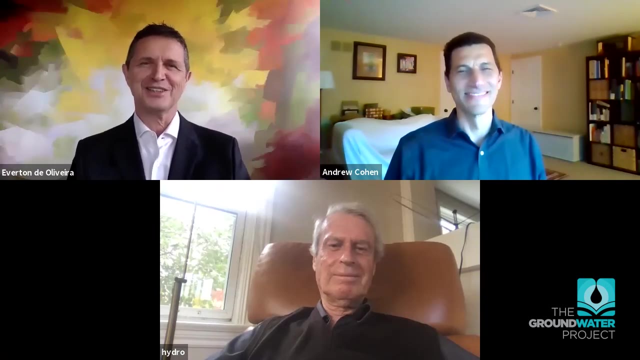 You just have to know what head is and Darcy's Law, and then you can start to actually learn about groundwater. Perfect, I can tell you I could do the exercise, so anyone can do it. It's, it's this simple. 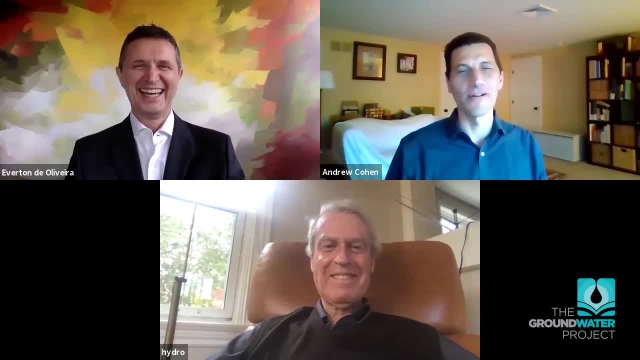 Well, I can you know, I can tell you that I've come across a couple of very experienced hydrogeologists that got stumped on some of the most fundamental questions, And it just goes to show you that I mean, certainly these people are skilled and they 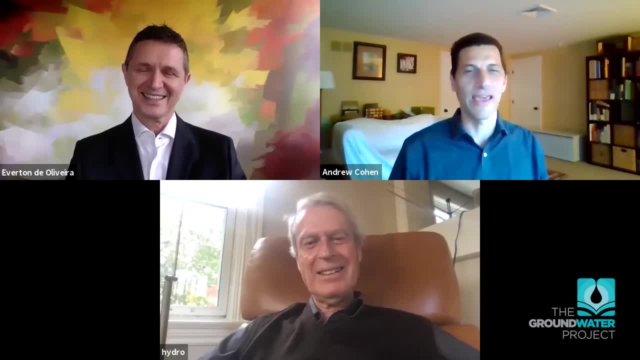 know what they're doing, but there are little subtleties that are very important and can be misunderstood, And I would just second John's point about the pondering part of this. You know that's something that we had in mind in developing this book. 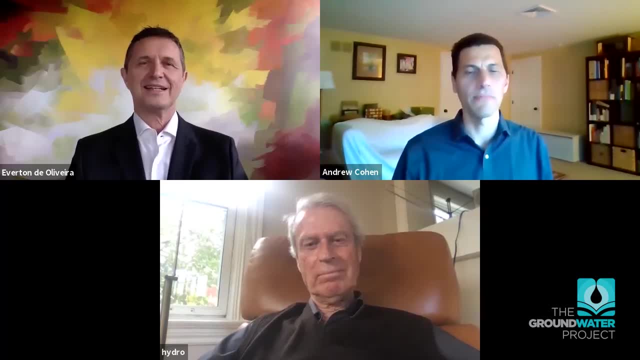 We want the reader to go through to learn, But at each week We continue to read, We continue to reiterate concepts and make reference to figures and things that were spoken about in previous sections of the book, And also we continue to ask the reader to ponder a problem. 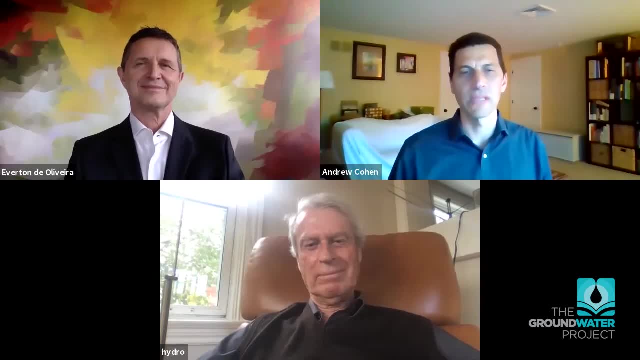 So a particular example problem is really requires the reader to think about it for a while. It's not a. it might get to the point where they can answer it easily, but they really need to ponder it. That's one of the the aspects of hydrogeology that I think is most satisfying is to ponder.